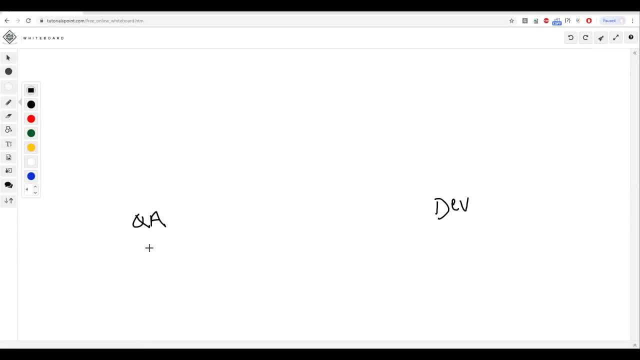 we have a QA team, like quality assurance engineer, all QA team we can. quality engineering team, we can call it is- and between these two teams there is one more team called as a DevOps, so DevOps development operations team. so what exactly these people roles are, we need to understand. so the developer. 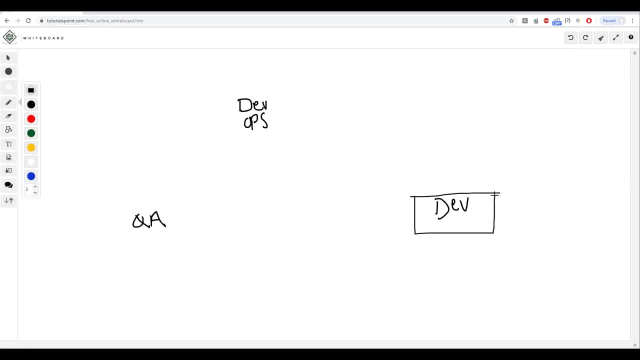 basically, will develop the code. so there are multiple people will be there, or multiple developers. they will write the code based upon their requirement and design and the QA people will test that code- not exactly the code. so, developer, I will provide the bill to the developer QA team and QA team will install that build on their environment and they will start. 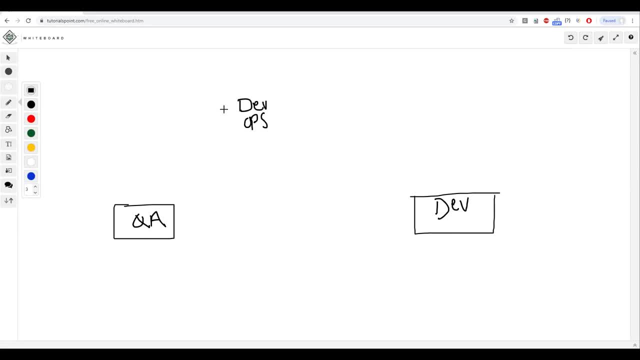 testing it according to the requirement and what DevOps team will do here. so DevOps engineer is having their own responsibilities, so they will do certain tasks from developers as well as QA engineers. so what exactly they do is so at the end of the day, developers- they check in their code in the 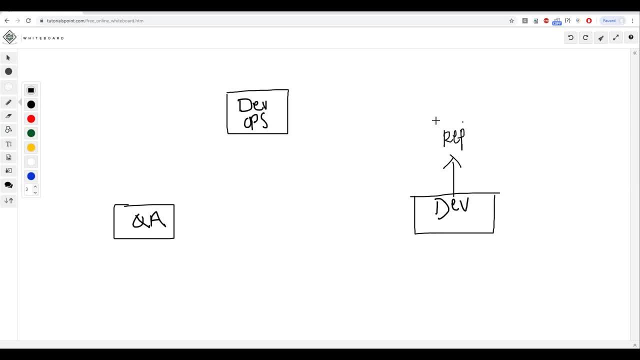 common repository. so because there are so many people will be there and they write the code based for different functionalities or different features of your project, so they will keep all the stuff in the repository. now what DevOps engineer will do is they can get that particular code and the first task they 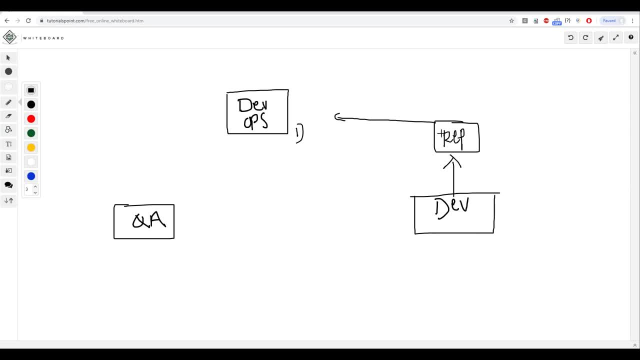 will do? is they will. they will create a build process. so, based upon that program, they will do some build process. now we'll see how we can do this. so here this is. first operation is a build process. they will build that, a particular software based on the program. that is a development task, basically, but 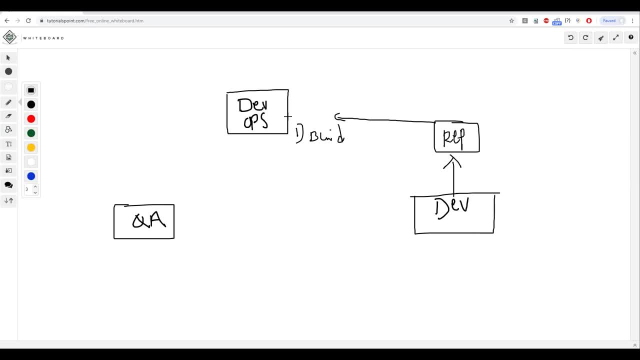 DevOps team will do that. they do complete automation process here to creation of the build and the other side from the QA side also, we write some automation script, basic automation script, to validate the build stability. so there comes under sanity as well as moat test cases. and as soon as 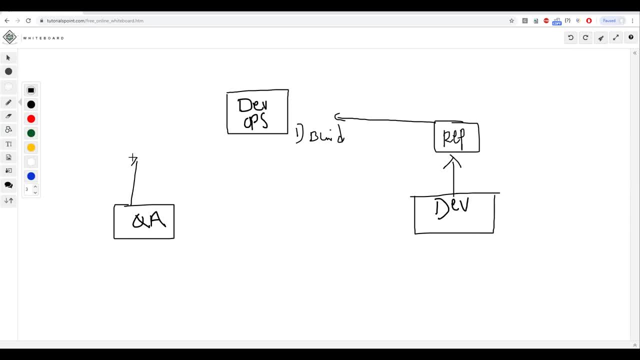 we have done basic automation stuff. we will also keep our automation script in the common repository, okay, and from there devops team will get that code. that means our automation script and that particular code will be executed on this particular build. so that is called as a test, okay. so first they will build that particular software. 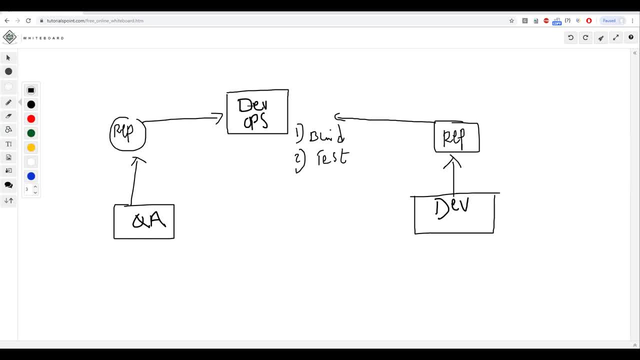 based upon the code they have checked in, and the other side, the devops name, will get our code, automation code, and run the test on that particular bill. so between these two processes there will be one more process called as a deployment and deploy. so deploy is nothing. 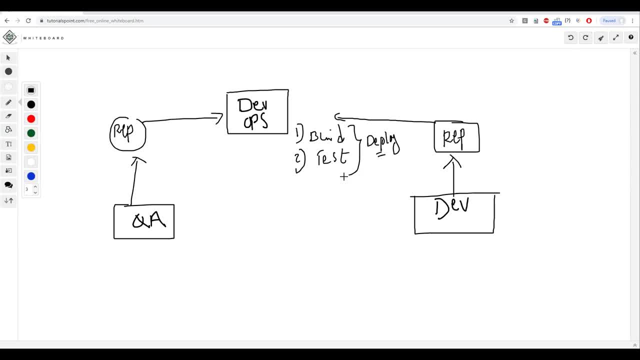 but a process of creating the build and testing. after that we need to test. so first we need to deploy the code in the environment and then they will build the software and then we perform the test. so these are the main activities. will be done by the devops team. okay, so deployment. 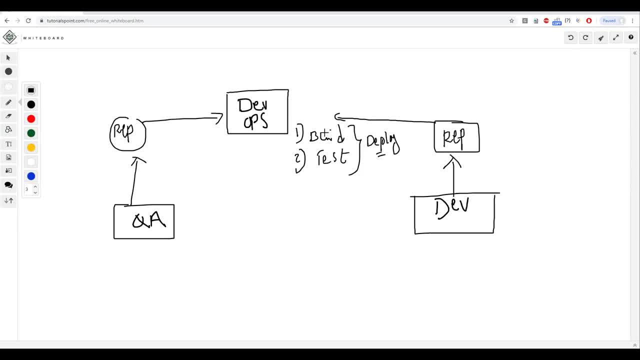 in the sense here this deployment means they'll create the build based upon the code. that process is called as a deployment and once the code build is done and test is completed here and to complete, uh, to do the rest of the testing like functional and other testing, so we will get that build from. 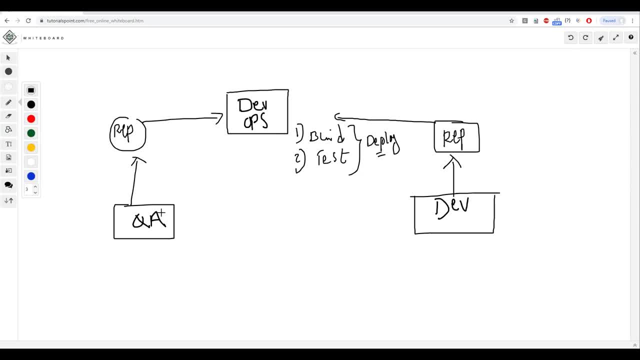 devops to q8 environment. we will download that, build and install that into q environment and then we can continue the rest of the testing. so the basic validation will be done in this environment itself. so devops is responsible for that. so mainly devops is uh, not a specific uh skill set, so they are having 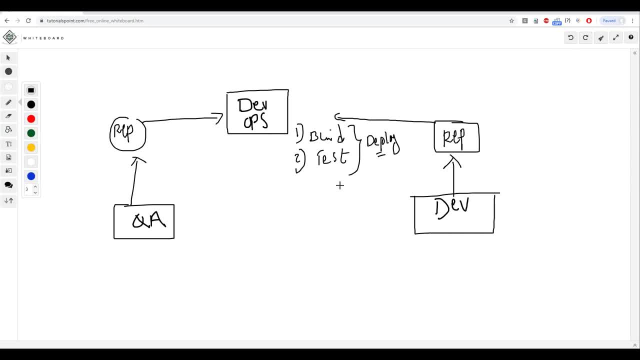 separate, separate skill set. like, let's say, they do some infrastructure automation, they do all activities automated. okay, this is just one time job and they keep on monitoring all these things are going fine or not. so this is basically a team, not a kind of a technology. it's a team. 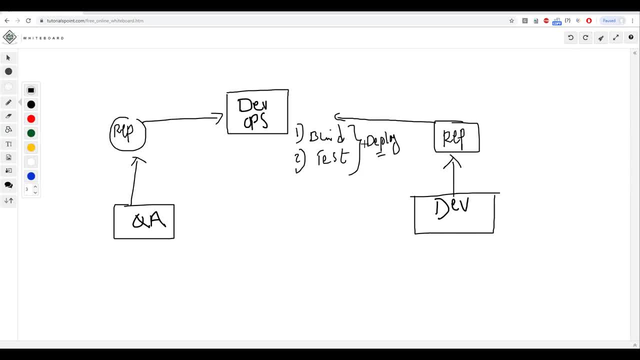 so the team is responsible for uh building, deploying the build, building the build and then testing it. so basic things will be done here itself and once the build is successfully done and uh approved then we can get that build satisfied or approved build. then we can download in the qa environment and we can start testing. 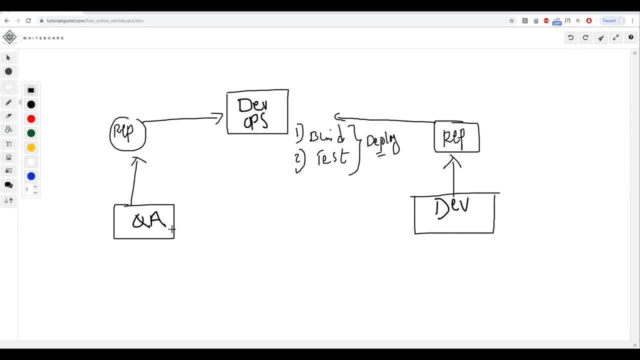 so this is a whole process. now, here dev as well as qa working together, uh, the developer will provide the programs at the end of the day, and here building deployment testing will happen, and again next day morning the bill will be ready and the bill will be approved. 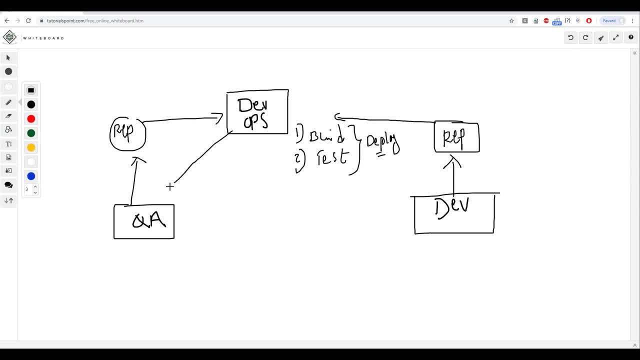 and then successfully pass and then create the download, the particular build, and start testing. so this process is completely called as a continuous integration process: developing the code, building the code and then downloading or deploying and testing the code. so this particular process is called as a continuous integration process. this process will happen between: 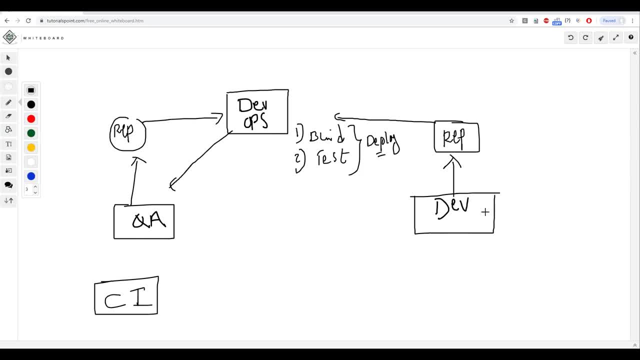 development and qa teams. okay, so at the end of the day developers will check in the code in the common repository- we can just call it a git repository- and here also tester will follow the same thing, and they will. at the end of the day they will put all the code in the common repository. 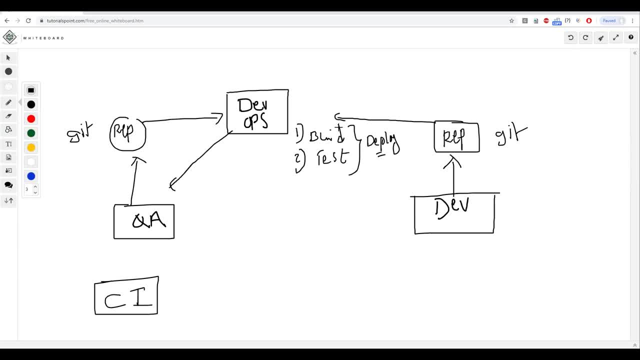 from there the devops team will get it and create the build through deploying process, and from the qa team also, they will get the automation code and they will execute that automation and, uh, that, test it. the basic testing has been done here and then bill will be ready the next day morning. qa can? 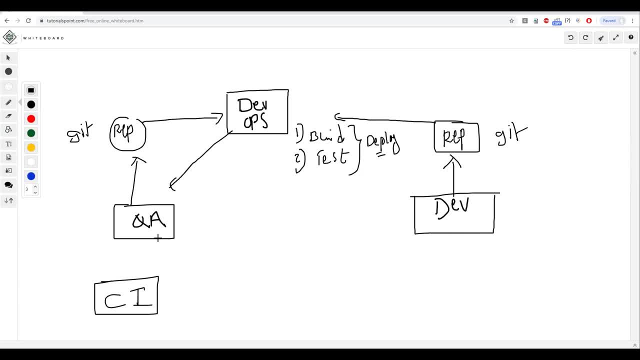 download the build and successful build and rest of the testing will be continued. so in the continuous integration, qa and developers will involve more. okay, this is called continuous integration process now. so these things will happen automatically. so they do complete infrastructure automation. so to do this they will use certain tools, like jenkins is the very best example tool. 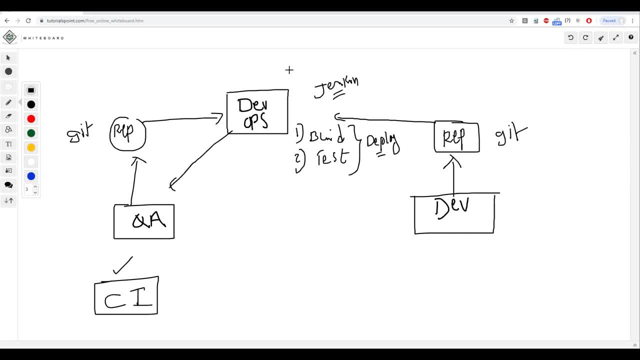 so jenkins is very popular tool which is available to perform continuous integration and continuous delivery. so this is a ci tool against a ci tool. so this is the one side. so continuous integration- now what is continuous? and delivery. so what is continuous delivery means? so, apart from this, so this process will happen between qa and dev, so getting the build and 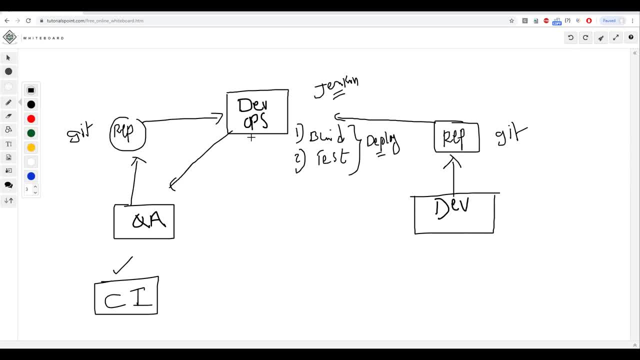 creating the, getting the code and creating the build, test the build and again deployment. here is a continuous integration process. so this is a continuous integration process. now there is one more process called continuous delivery process. and what is a continuous delivery means? it is just an enhancement of continuous integration. so, in addition, after getting the code, creating the, 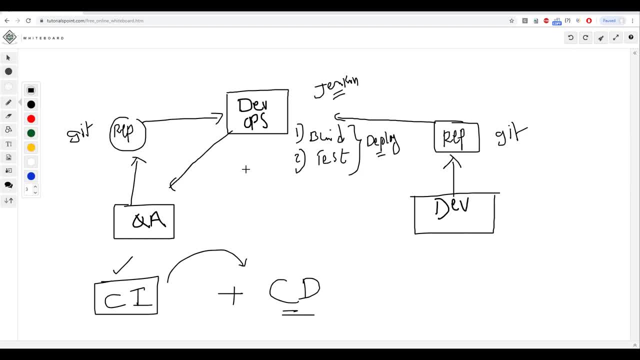 build, testing, the build okay, and these things will continuously happen. so, apart from these steps, there will be one more step called as a release process. so this is a continuous integration process. so as soon as the build is done, testing is completed, immediately it will go to the next level. that's a 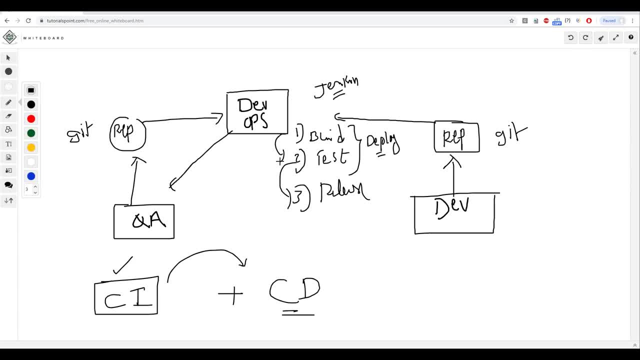 release process. so here build is created, testing is also done. as soon as the testing is completed, we release that particular bill to the customer. so this is the additional step. so here this is called as a delivery process, continuous delivery. we'll get the code. build that, uh, based on the. 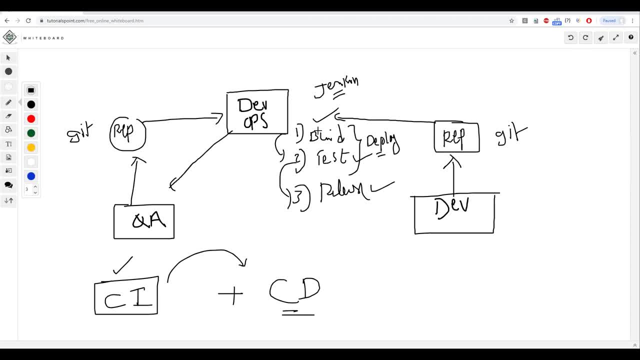 code, build that software, test the software and release the code. so so this is a continuousBLU-DVD: the software to the customer. again one more, again, implement new functionalities, again and again, build that code and test that code, again release. so this process will happen continuously and here. 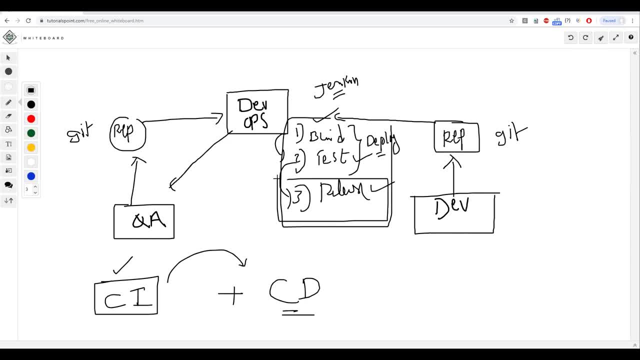 the delivery is also there, releasing in the sense it's a delivery, so continuous delivery is also happening, so this whole process is called as a continuous integration, continuous delivery process. okay, so to automate these activities, devops team is the main responsibility, but they use certain number of tools here, like Jenkins, maven, docker, and many more tools are there so they will use. 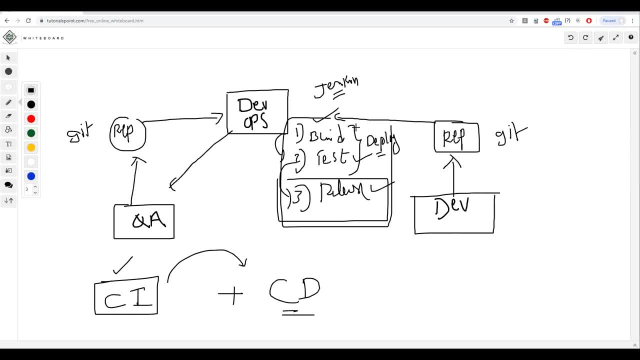 certain tools and also write certain kind of automation stuff to establish kind of infrastructure. and they do everything is automated, okay, so continuous integration and continuous delivery. so to do this they use a tool called as a Jenkins. so to do these processes like deployment, build, test, they have to. 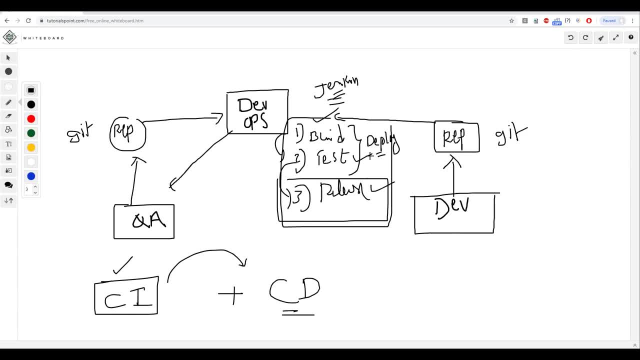 create number of jobs. so every activity is a job, as a build is one activity which involves a lot of jobs. job is nothing but an event or an activity. so if you want to create a bill, they have to go through certain number of events or they need to run certain number of jobs. and similarly, if you 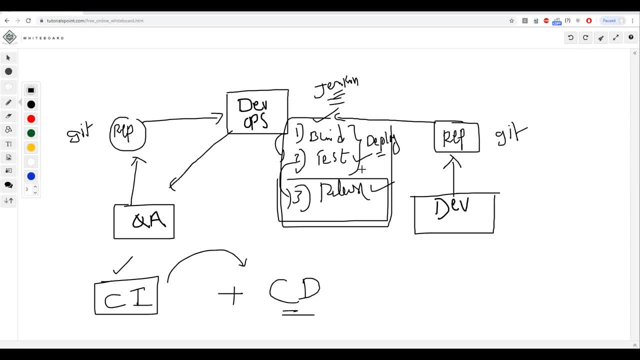 want to test that build, we need to again run certain number of jobs. and for deployment- Deployment- we need to run certain number of jobs. Similarly, to run the release process, We need to run a certain number of jobs. so every activity involved certain number of Processes, a certain number of jobs. 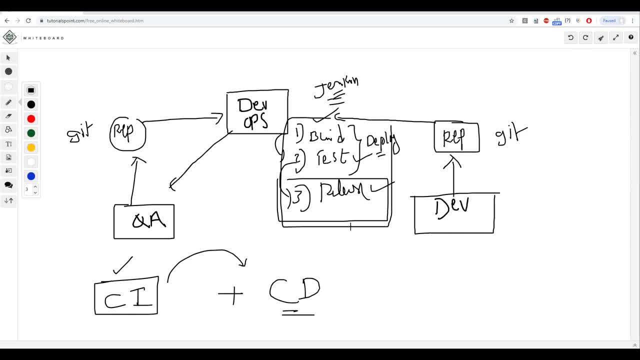 okay, so this, all the stuff, will be taken care by a single tool, which is Jenkins, and By using Jenkins we can automate continuous integration and continuous delivery process. Right, So here to automate this process, every activities depend on some other activity. suppose Deployment is one activity, or build is one activity and testing is another activity, release another activity. 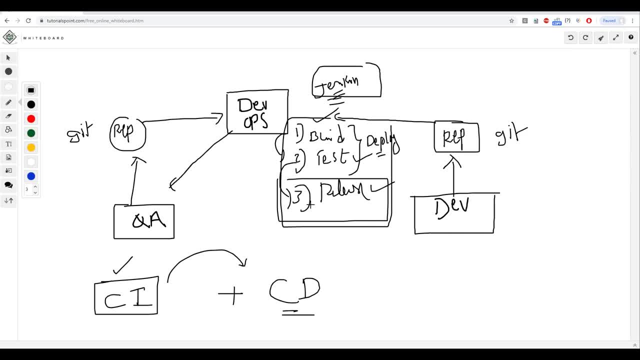 So every activity is depending on some other activity, right? So if you want to perform these activities, we have to follow certain process, or sequential. let's say, first we need to get the code from developer and then we need to build it and after that. 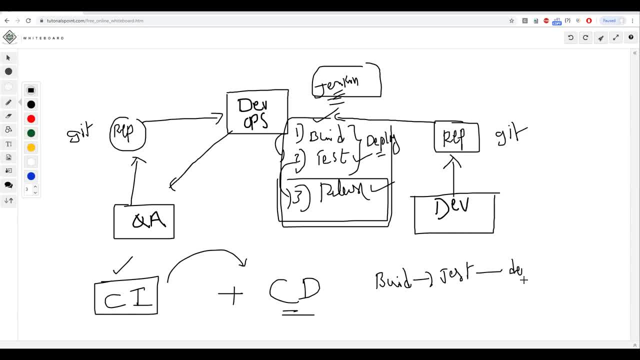 We need to Test it, after that We need to do a deployment and after that we need to release. so we need to go through certain process and Every step is depends on a previous step. So every step again we need to run multiple jobs. So here: build jobs, test jobs, a deployment, a deployment task or deployment jobs, and release jobs. 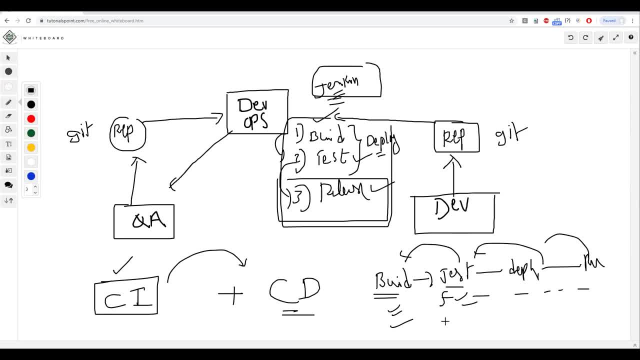 So job is nothing but an event. So we need to do a lot of, we need to run multiple jobs in every phase and after that, once after, everything will be completed and finally the software will be released and Software will be delivered. So which includes continuous integration as well as continuous a delivery. 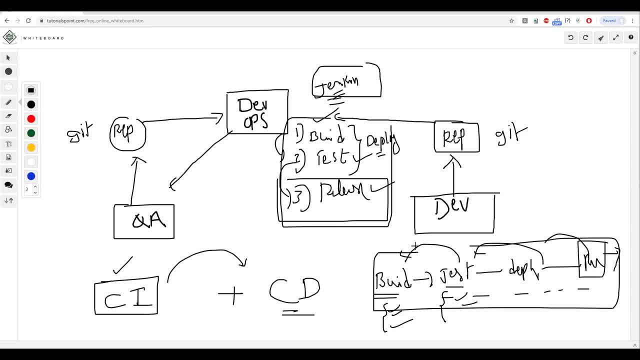 Okay, so this particular process can be achieved by using Jenkins pipeline concept. So creation of the build, testing, deployment and then release. so these things Continuously we can do by using Jenkins pipeline concept. Okay, Now let us talk about Jenkins pipeline. So let me just say a small presentation. 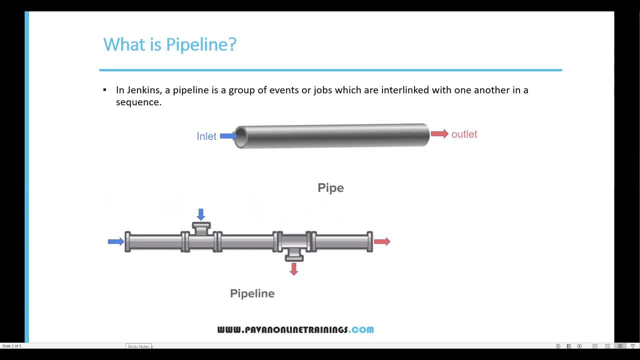 What exactly Jenkins pipeline? so first let us understand what is pipeline. So in Jenkins a pipeline is a group of events or jobs Which are interlinked with one another in a sequence. So what is the pipe here? Normally pipe is having some inlet, some outlet. 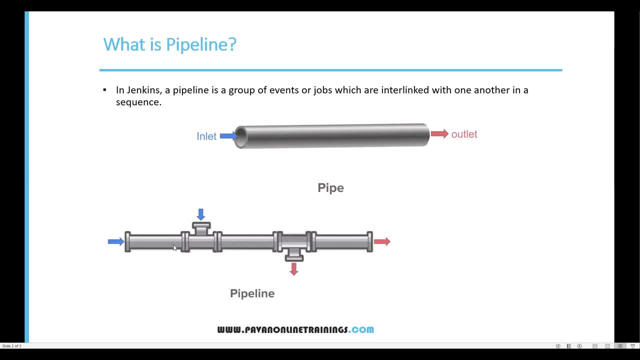 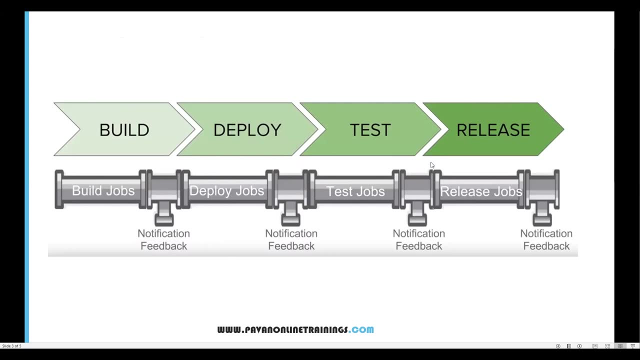 So again, the pipe is divided into multiple sections and every section Is having a different type of actions or activities will be done. So if I just understand this particular process, it will be like this: So the in Jenkins, the overall process, the pipeline process, is divided into four things. So build: 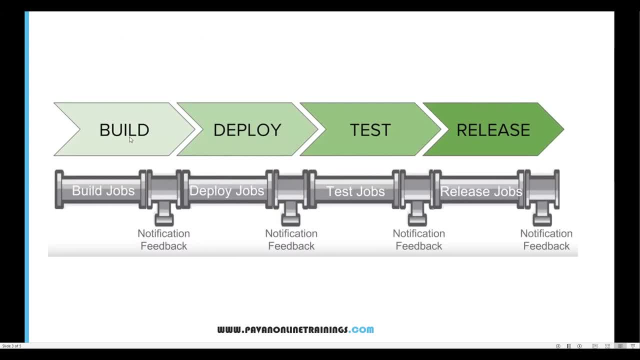 deploy, test and release. So these are the four different phases. So the first one is from the development. they will get the code and they will do the deploy. so will Can be created using deployment process. So first they will build it and then they will do the deployment and 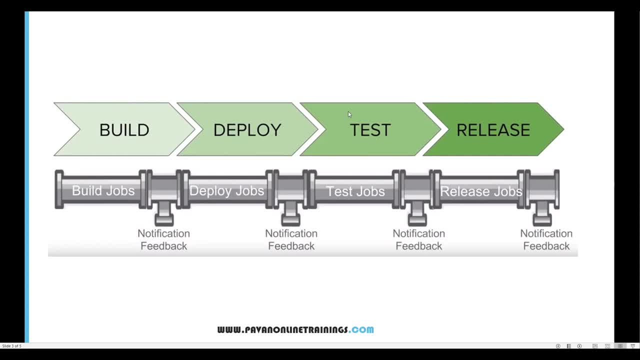 Then we do the test and then release. so the entire pipeline is divided into four different parts. One is build, deploy, test and release. so build is nothing. but here they will run certain number of build jobs and those jobs will be created a build and on the deployment they will run different deployment jobs and they will do the deployment process. and 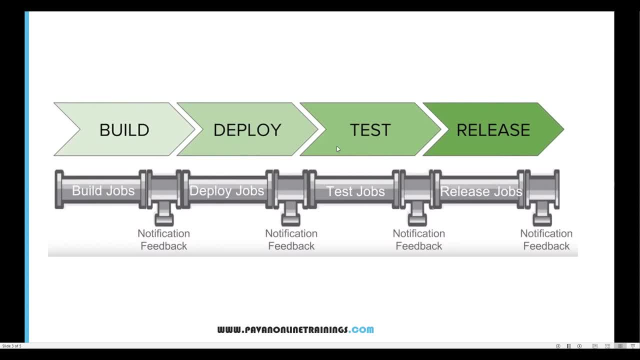 the testing we will have a number of tests jobs, so they will test our software which is already built and deployed. once the testing is completed, we release the software, and here we need to run set a number of release jobs. so what exactly these jobs will do is the jobs will make. 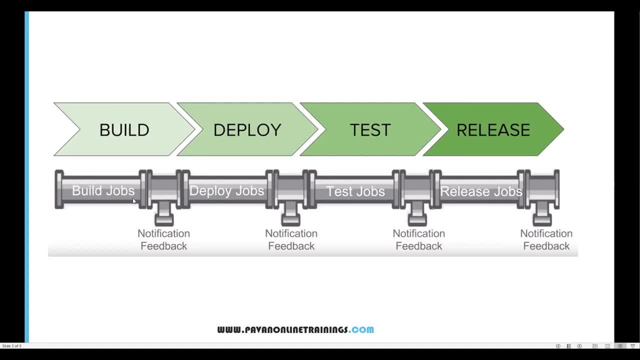 sure everything is goes well. so the first these jobs will responsible building it, deployment, and testing and releasing. so this is a continuous process and dependent process. deployment is depending on the build creation, testing is depending on the deployment, releases depending on the testing. okay, so these things will happen continuously and every activity having certain number. 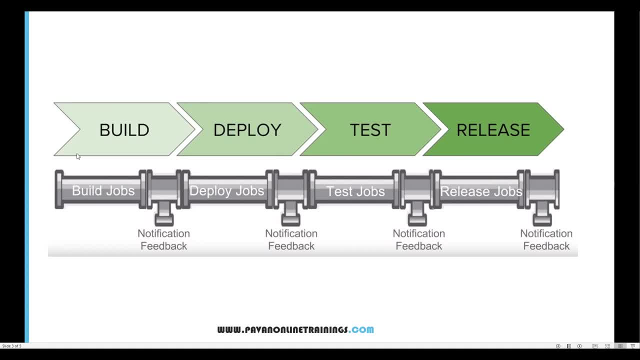 of jobs. so this is called as a pipeline in Jenkins. so these activities we can define, we can create and once you start initialize, or once you start run this particular pipeline, all the activities will run sequentially, one after another. at the end we will release the complete software to the customer. 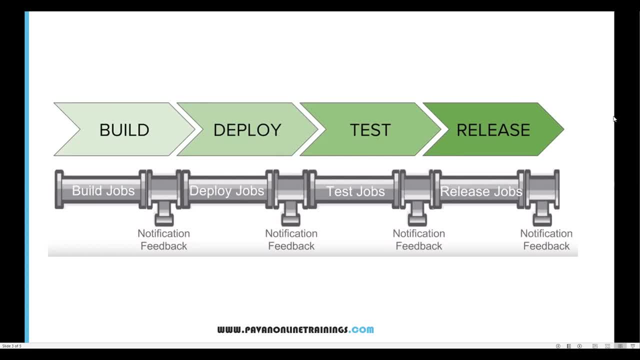 you. so this is a whole continuous delivery process. so build, deploy, test and release as per the Jenkins. this is a process now. so if we just see how to set up build by how to set up build pipeline in Jenkins, so now we will see practically how we. 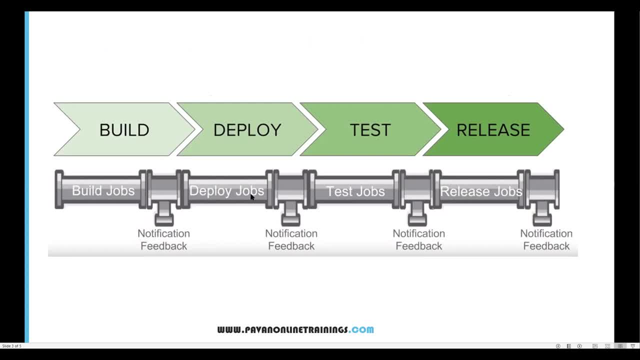 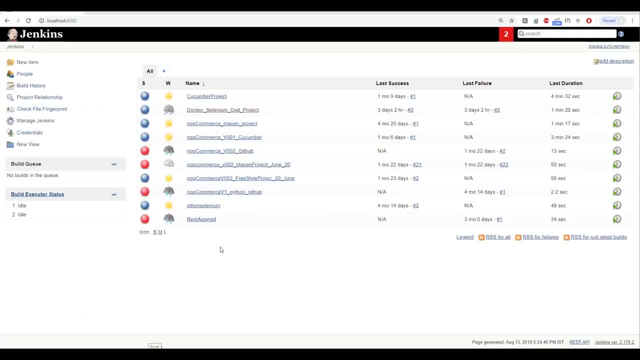 can set up all the stuff and how we can define this, how can create a pipeline and, through pipeline, how we can automate these activities. we will see practically now. so to do this, I'm just opening my Excel Eclipse. I am opening my Jenkins, so this is my Jenkins application in my Jenkins. 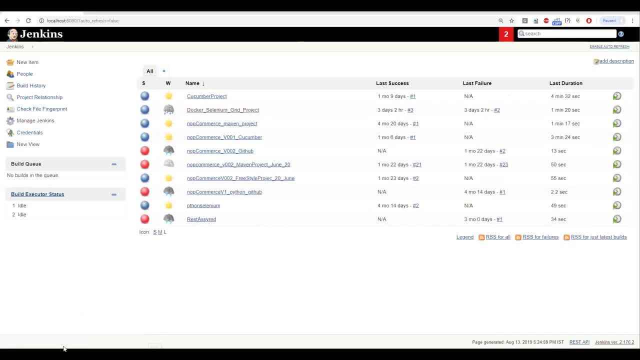 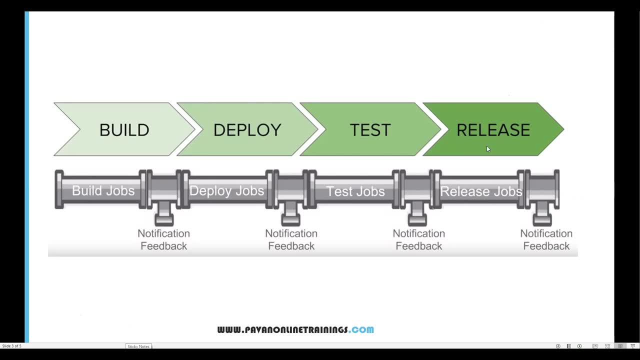 package. first I will create a different jobs. so again I said earlier, every phase like build and deploy, test and release, having different number of jobs, and these jobs we need to execute sequentially, one after another, through pipeline. okay, now let's go to Jenkins now. first of all, we need to house at a 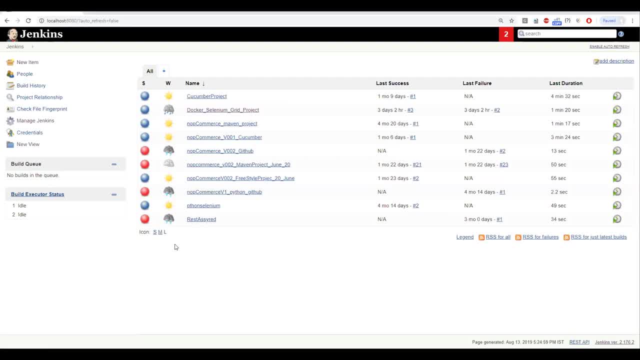 number of jobs which are related to multiple sections like this. okay, these are theADEc, now let's go to Jenkins. now, first of all, we need to house at a number of jobs which are related to multiple sections. вкус, you think now we gonna shut off? you have tried it. right now, this process sort of changes every single job, um, and if there is some kind of problem with domains related to» is what you see heresten, i'm going to open it up to let the SEO forces and initially toggle this process for you and 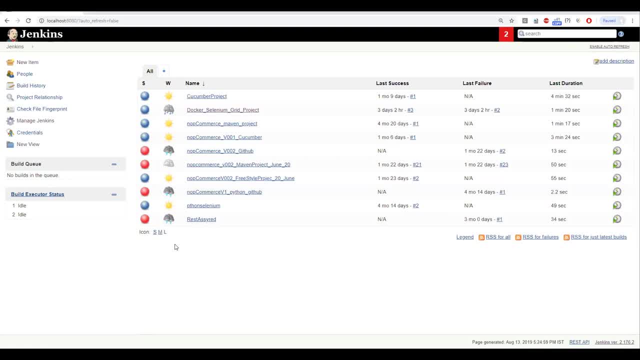 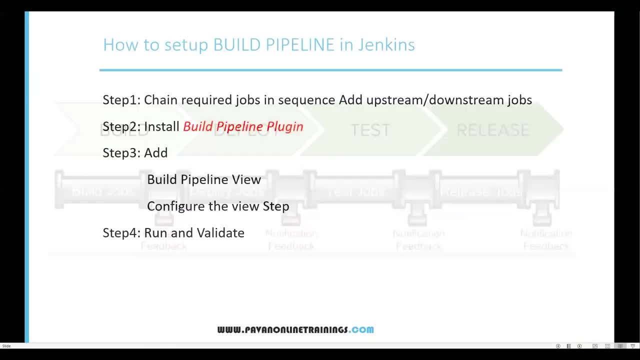 sections right, so that we need to create first, and after that i will integrate everything and then i will show you how we can pipeline that. so to do this, we need to follow certain process. so as a first step, we need to create multiple jobs which are related to multiple phases. 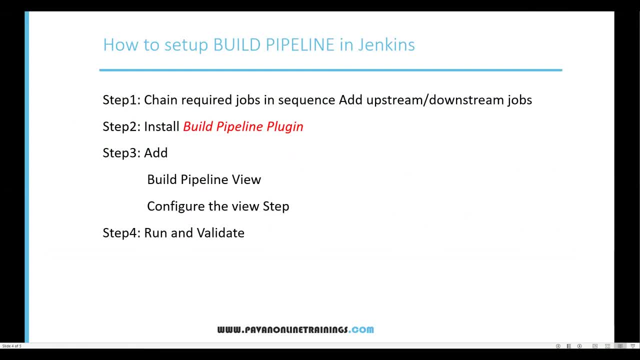 and again, every job will be created by using different type of commands. okay, so as normally in the devops team, you'll write a certain number of automation script to do that. so in my video here i'm not going in depth of that- how we can create all the jobs and everything. i'll just show 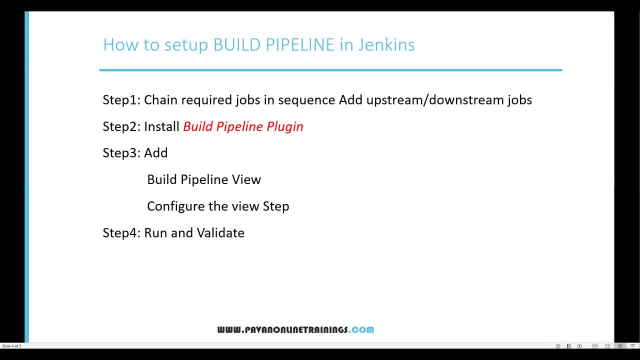 you how to create a simple jobs and how we can link them and after that, how we can execute all the jobs within the pipeline. so that's the main concept i'm focusing on. all right, so here we need to follow certain number of steps to build a pipeline in jenkins. the first step is: 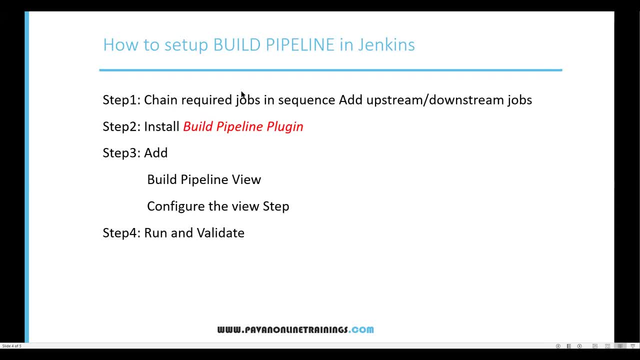 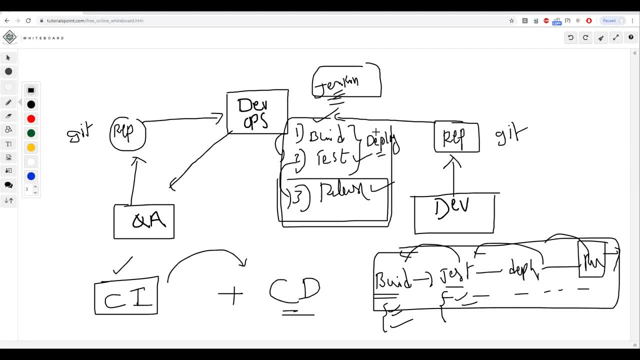 you need to create a pipeline in jenkins, and then you need to create a pipeline in jenkins, we need to create a chain which required number of jobs. so what is the chain is nothing, but here, as i said, multiple operations we are going to do right. first we need to deploy. first build, deploy. 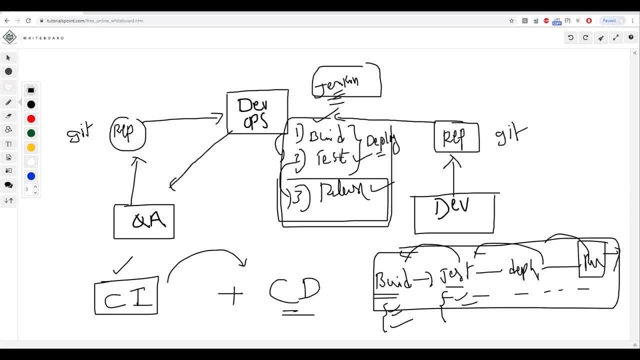 test and release. these are the four activities and every section we have multiple jobs. so first we need to create multiple jobs like this: one, two, three, four and so on. some of them related to build process, some of them related to testing, some of them related to deployment, some of them related 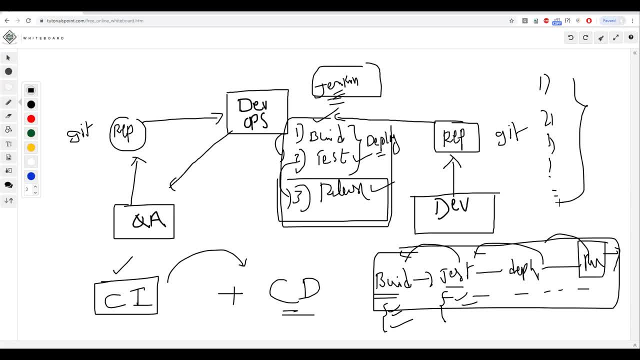 to release now we need to create a chain, which requires number of jobs. so what is the chain is? now, we need to link all of them because there should be some dependency. so if you want to establish some dependency, we need to link them right. so this is a basically called as a chain. 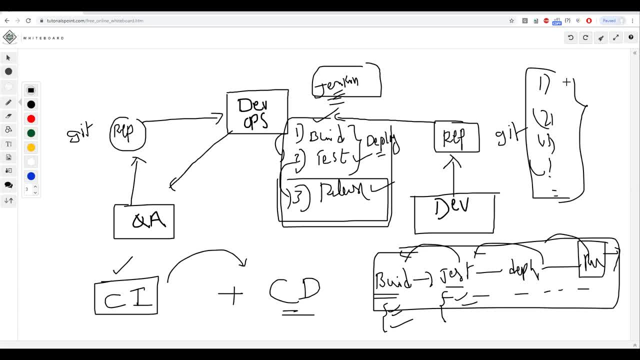 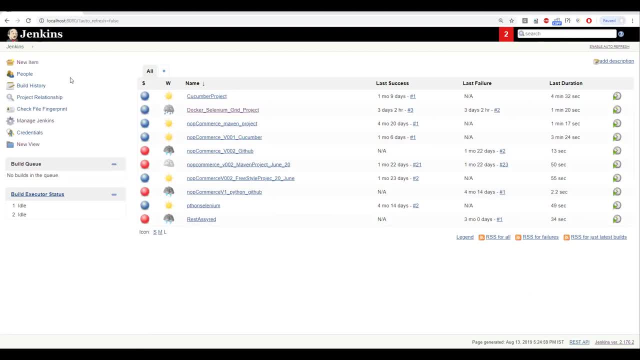 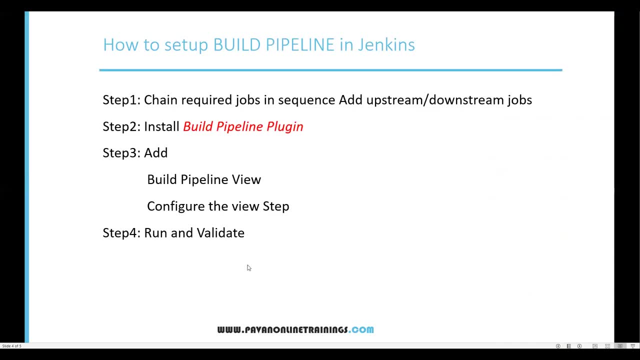 so we need to create a chain first of all. so for that we need number of jobs. so now let's go to jenkins. i will create multiple jobs here. so how to create a new job here? just go to new item now. here i'm going to create multiple jobs. as i said, we have a 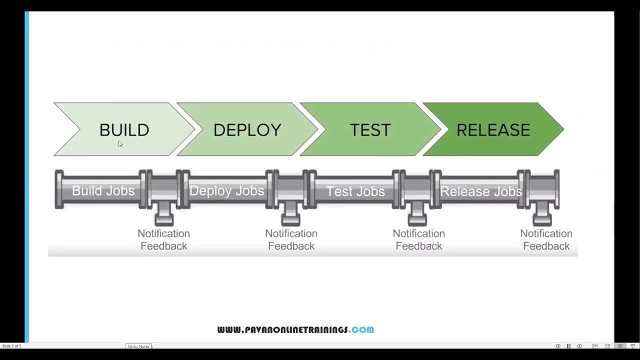 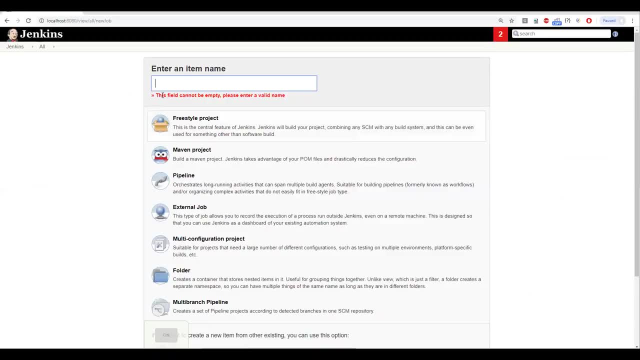 multiple phases- build a deploy, test and release- so every section can have multiple jobs. so for demo purpose i'm just creating one job in each and every section. so first one is a build section. so here i will create just sample build job. okay, so this is sample build a job. now let me just take the 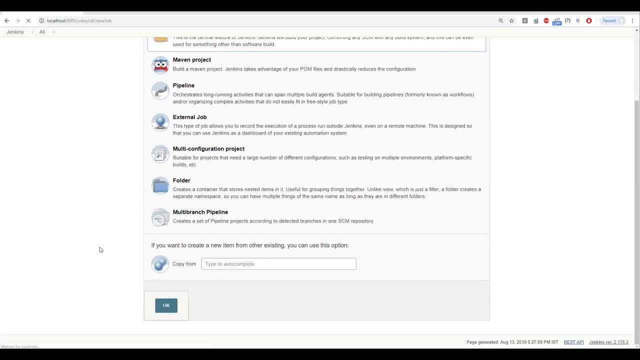 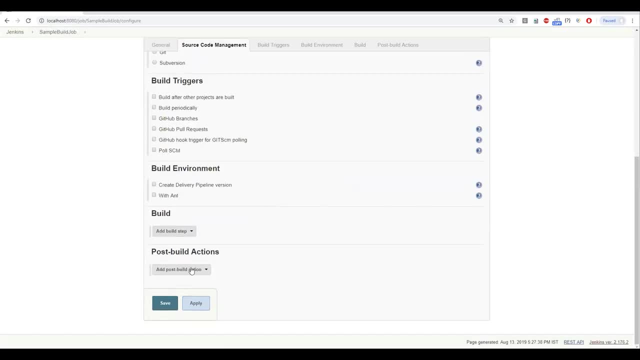 freestyle project for now and just click on ok, right. so now we need to add some configuration to this particular job. so i'm just going to add some configuration to this particular job, so let me drag them in here so we have your scale here again, you need to make it come out from here. 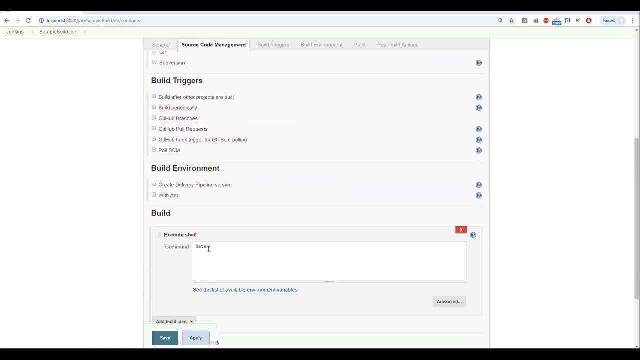 so let's do that. so let's take this marque. these are task clear Luigi. it's gonna quite enhance necessary things later. let's make this a little bit cooler, because if it was just the mobile data, but when the web is to be built right now, let me, let me copy and paste it there. 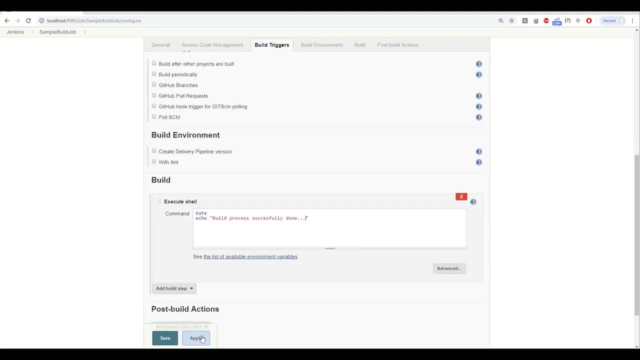 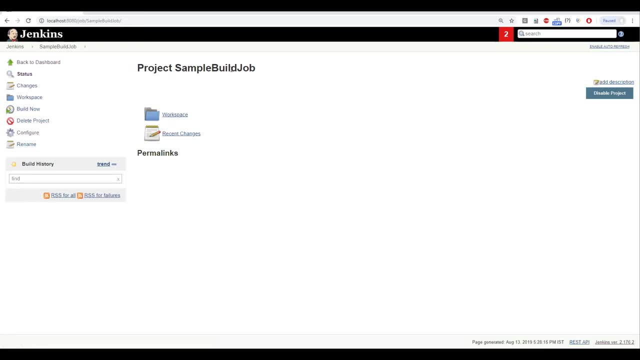 i can paste that, so let me copy that. changes to simple and local life as well. i'm gonna leave that already where it does now make it readable. are going to be a вот. this comes out exactly what i'm, and then save it, so just created a simple job. okay, that is a build job. i'm just naming it as. 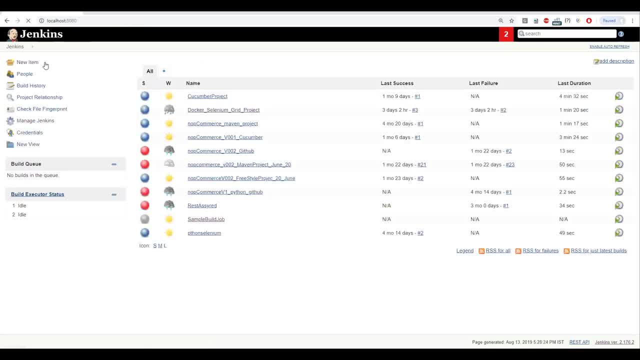 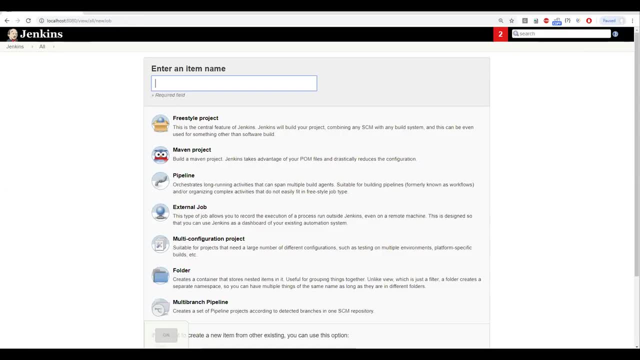 a build job. after that i will also go to again dashboard and then i will create one more job. go to the new item now. this time i will create one more job, which is deployment job. so let's say, a sample deploy job, sample deploy job. now i'll just create a freestyle project and then 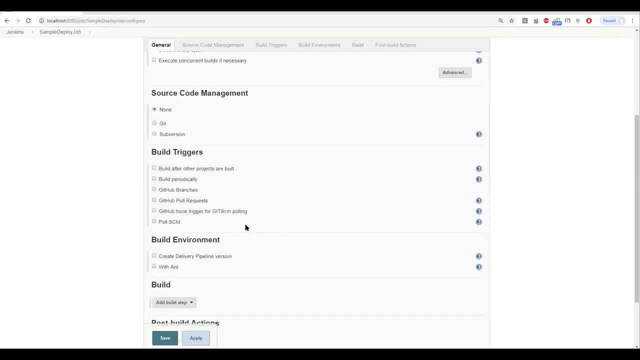 okay button. so again here, just go to build section. i'm just selecting windows, execute shell command and just i'll print some date here and i'm just writing the echo command. so but actually the devops engineers will write a lot of things here. each, each and every job will. 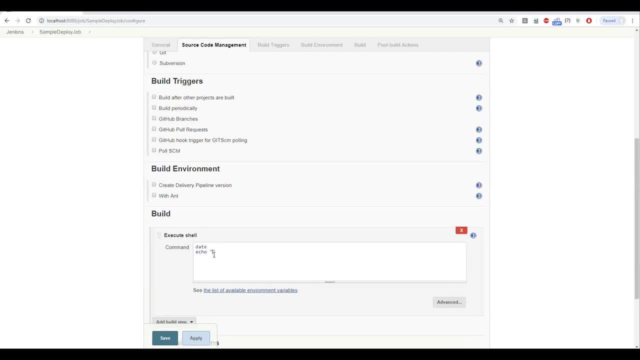 do a lot of activity, okay. so here i'm just saying: successfully. so this is which job it is, it is a deployment job. so i'm just saying successfully. so this is which job it is, it is a deployment job, right? so let's say: deploy job, deploy job successfully executed, deploy job successfully. 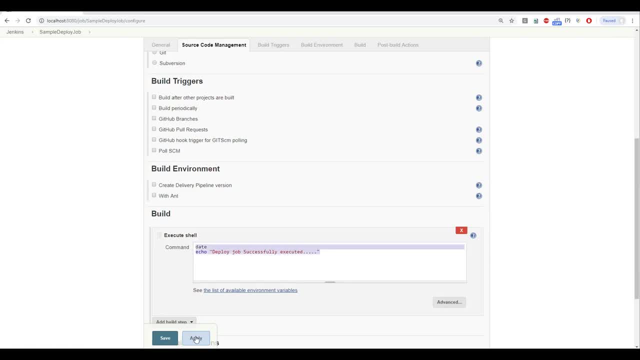 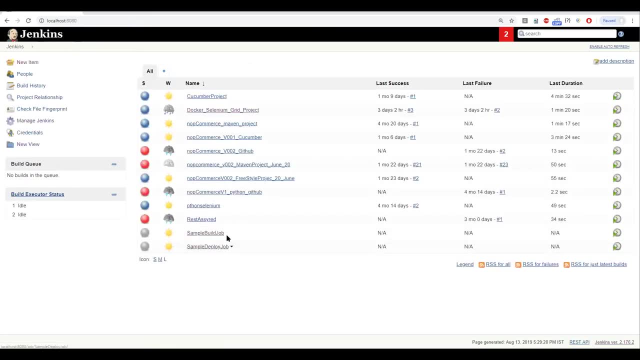 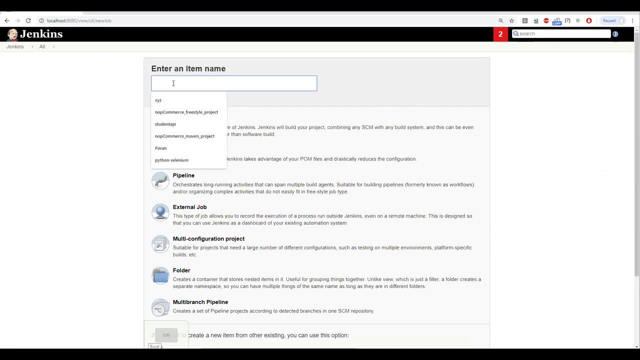 executed all right, so now, similarly, i'll just apply and save. now i created one more job again. go to dashboard now. so far, we created two jobs: build job and deploy job. so what next? we have to create a test job. now let me just create one more new item and i'll name it as sample. 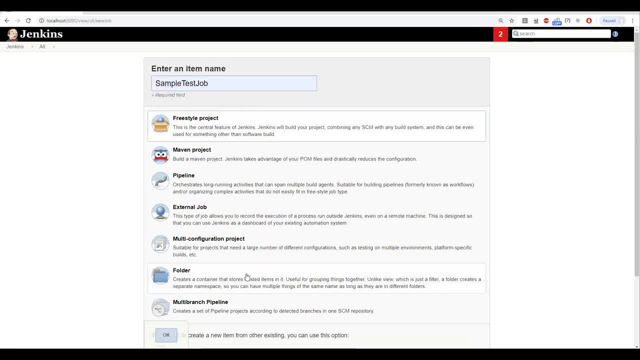 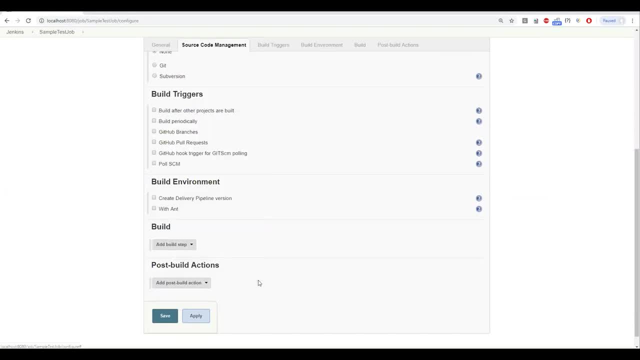 test job. now again, take the freestyle project and okay, now come to build section. so come to build section, execute shell and just put the date. and here this is test job, test job completed, executed and then apply and save. so far i created two, three different jobs. go to. 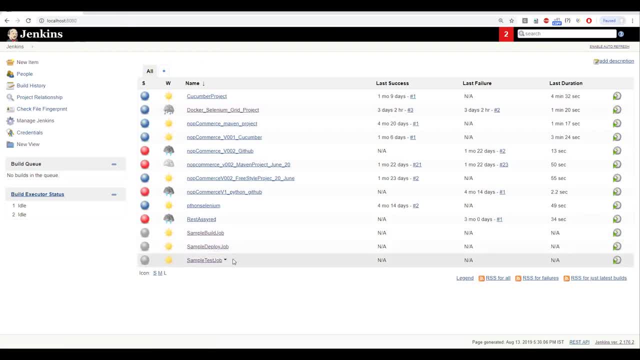 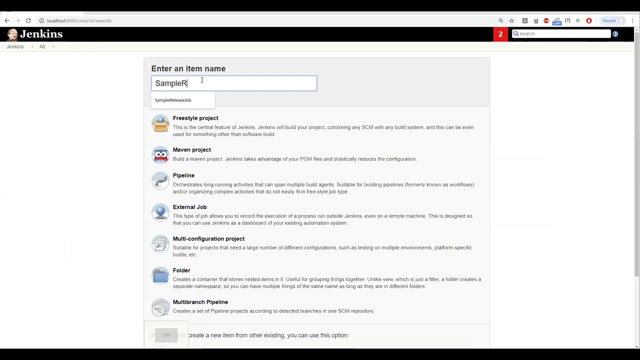 dashboard again. so sample build job, deployment job and testing job- right, so i'm just going to. so one more is there, so that is called a release job. so i'll create one more job which is related to release process. so go to the new item and here i'll say sample release job and go to select freestyle. 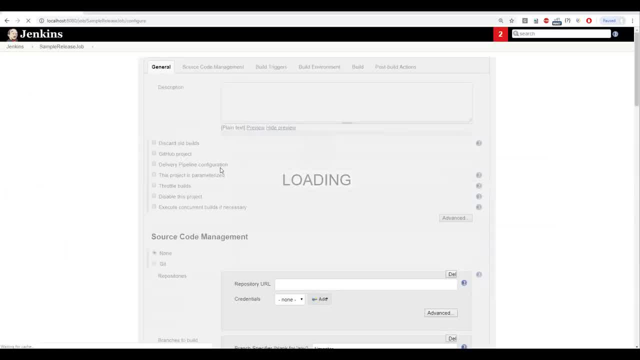 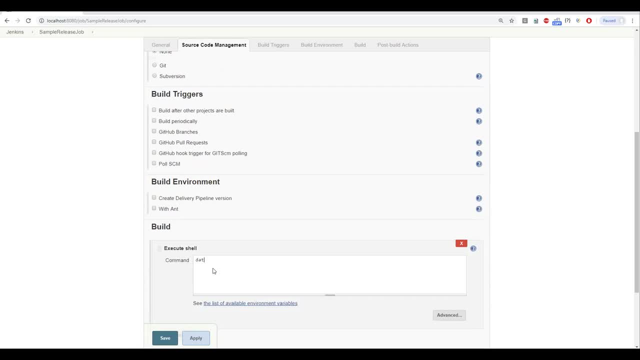 project. okay, now here, go to build section execute shell. i'll print the date first and then i'll just write some echo, comma echo just print the message: so this is a release, release a job, right, so release. job successfully completed, right, so now apply and save. so just go to dashboard and now we can see. 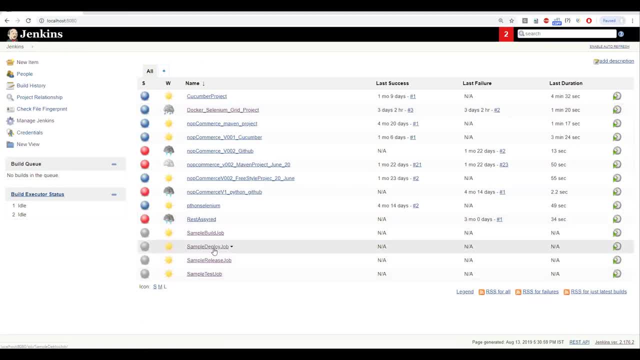 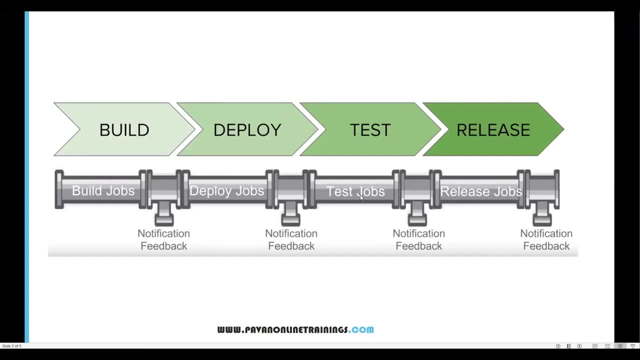 there are four jobs i have created. one is deploy, build, then deployment, test and release. so this is order. so first build job, then deployment, then testing jobs and release jobs. so it will go sequentially and everything is a dependent. now how we can link together. that's a first step. so we need to create a chain between them. so how to create a? 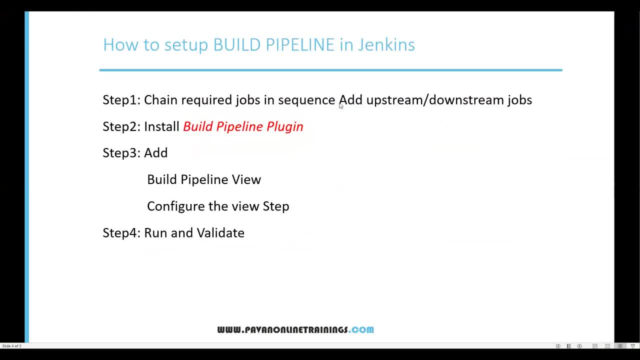 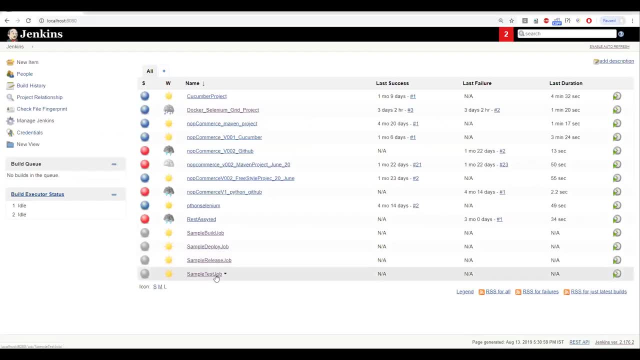 chain, so chain required jobs in sequence and add upstream and downstream jobs. we need to add. so what is upstream and downstream jobs are nothing but here. for example, let's say uh deployment job, so for this build job is a upstream job, okay, and uh release job is a. 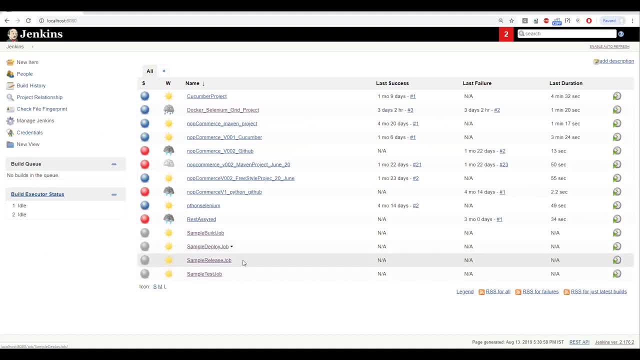 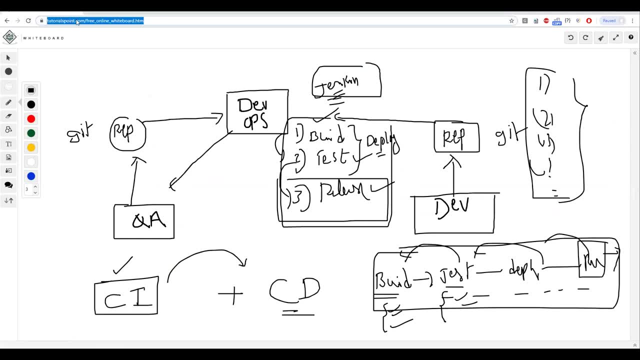 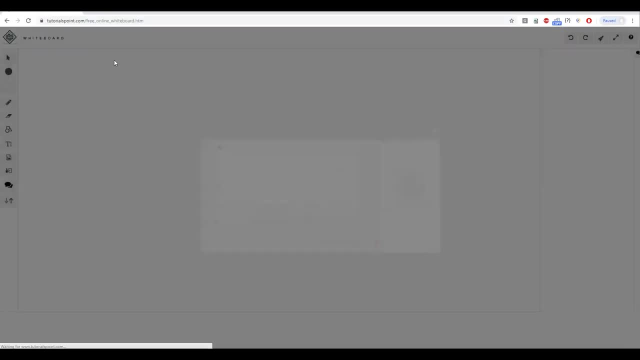 downstream job. similarly, for every job, there will be upstream and downstream job will be there. so now I need to link them, so how we can link it. so let me just open one more tab, so how to link them. so I have just created four different jobs, right? 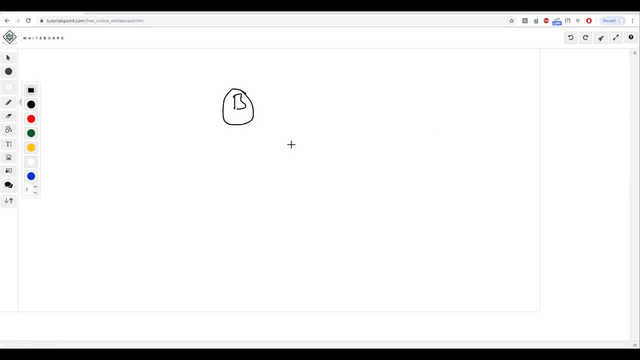 so first one is build, so build, and then, after building, then deployment, and after that testing, and after that really. so this is a cycle which we need to do it. so the deployment is depending on the build, testing is depending on the deployment and release is depending on the testing. so we need to link together. 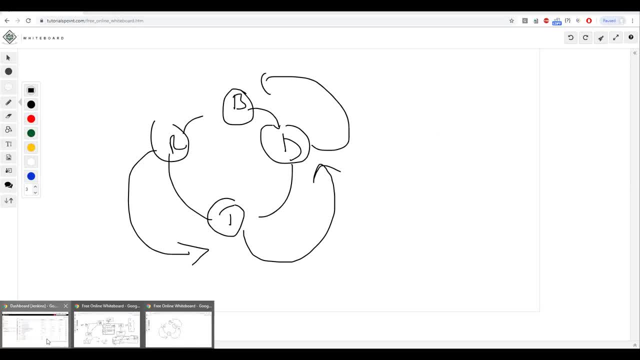 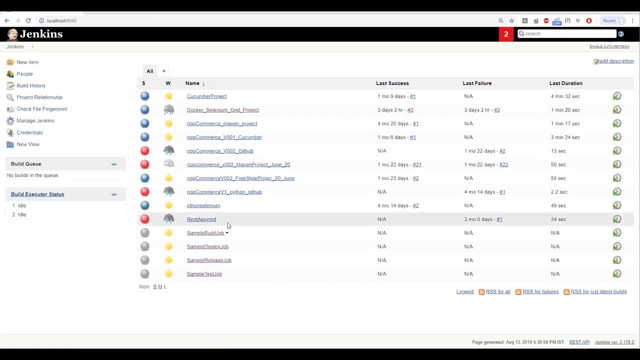 so how we can link it. now go to Jenkins. so the first job which we need to run is build. so for that there is no before before job is right. these are basically starting job right, so we no need to configure anything here. so after that sample deploy job should. 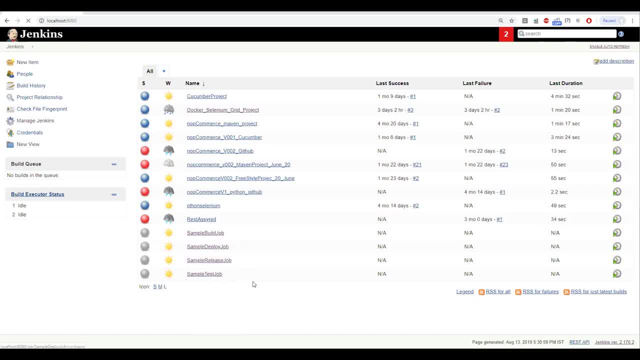 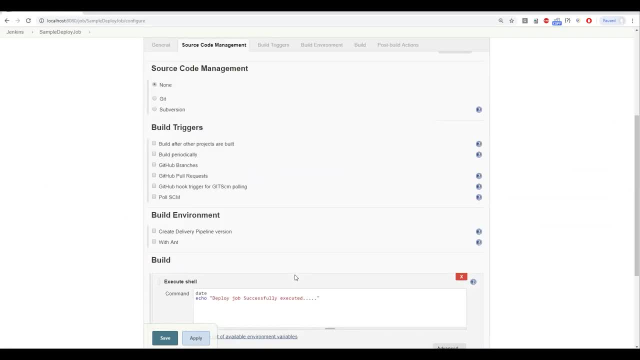 execute, so we need to configure it. go to configure. and before executing this job, I need to execute the build job, right? so here we need to specify that. just come down under build trigger section. you can see one option called build after other projects are built. built after other projects are built. 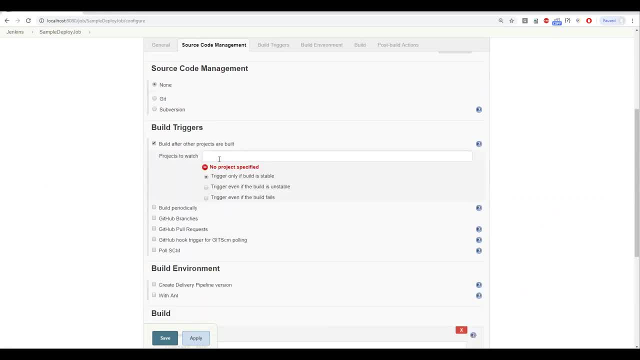 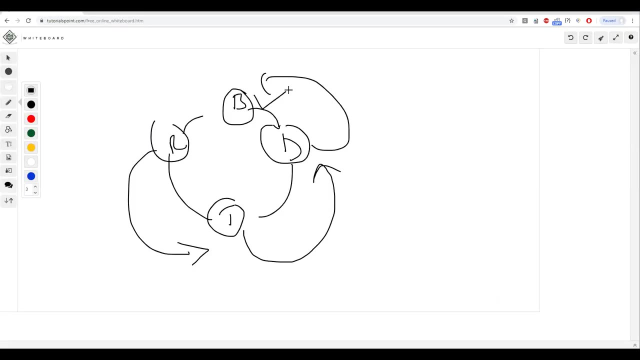 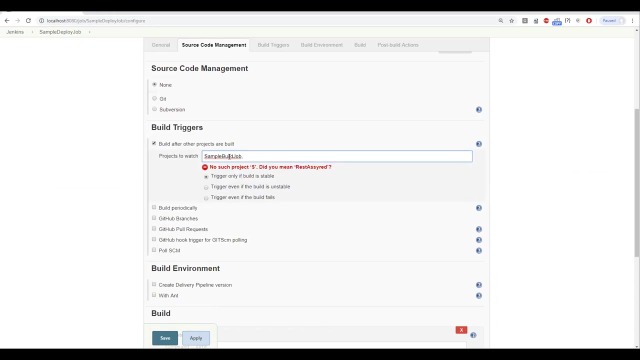 so just select this option, then it will ask you which which job you are expecting to complete before executing this particular job. okay, projects to watch? so here we need to specify that. so, before this, so before deployment, I need to complete the build job, so that I need to specify so, sample. so build a job, I need to complete sample. 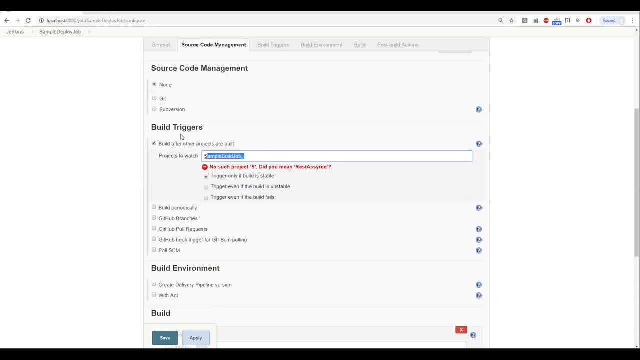 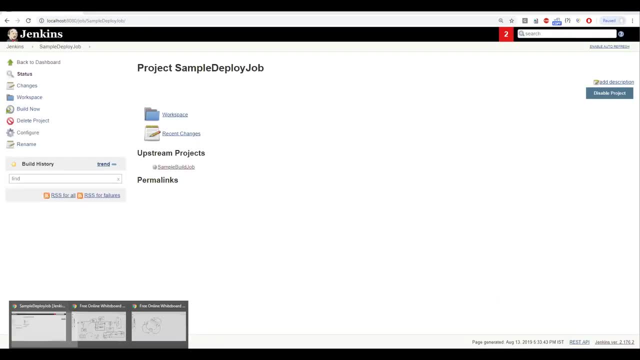 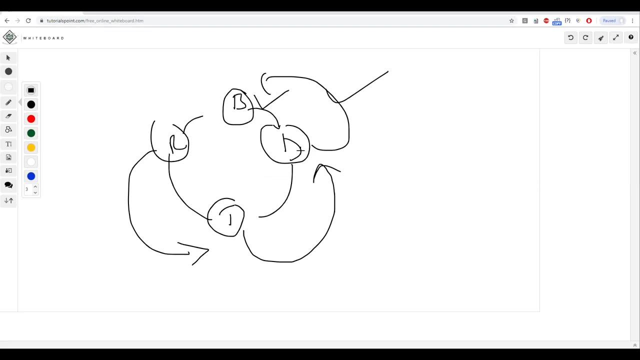 build a job I should execute before complete, before starting this one. so manual and simple'll have to be completed before starting this one, okay, and then it will start here: projects to watch and then apply and save. so this particular part is done now. the next one is a testing job. so if you want to execute this deployment job, 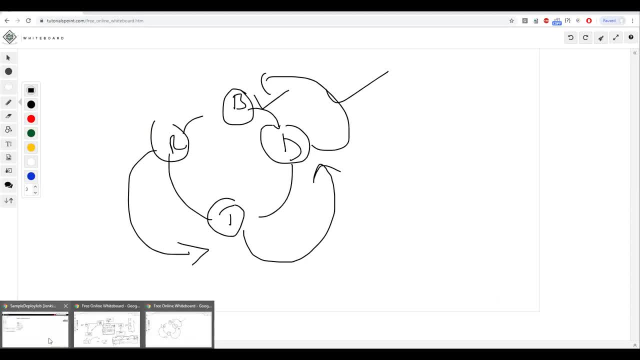 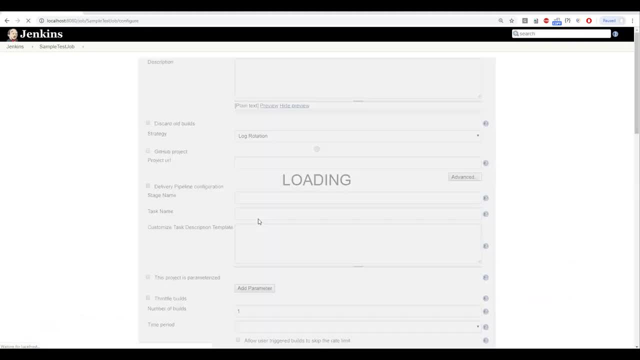 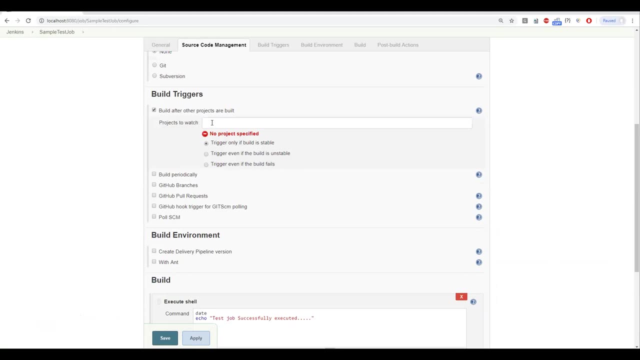 should complete. now go to the testing job, go to jenkins again, go to dashboard. now go to test job and do the configuration. so here just again come down, select build after other projects are built. now here you need to specify sample sample deployment job, because this is a testing job. so 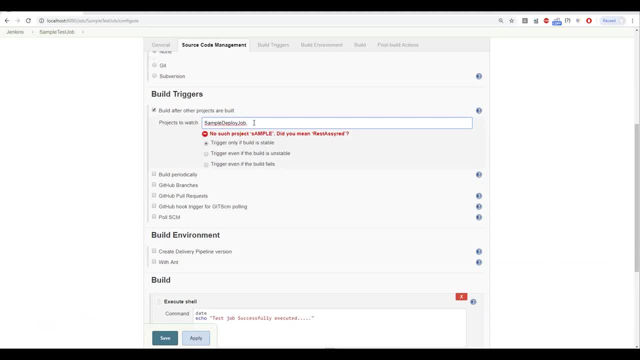 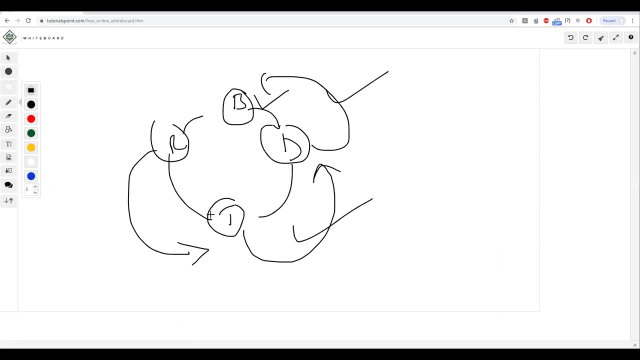 if you want to complete this, we need to run. the deployment job should be completed. so deploy job and trigger. only bill is stable. if the previous job is successfully executed, then this job will execute, then apply and save it. so now we have also done this particular part. now a release is. 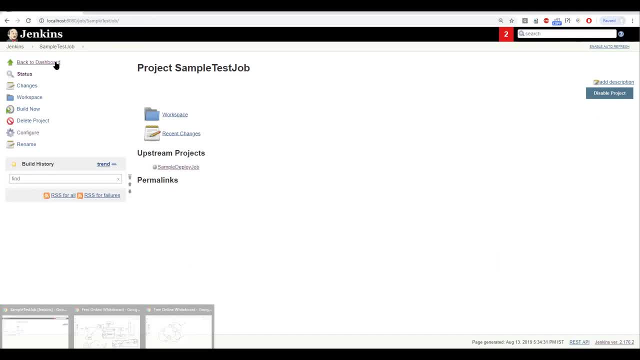 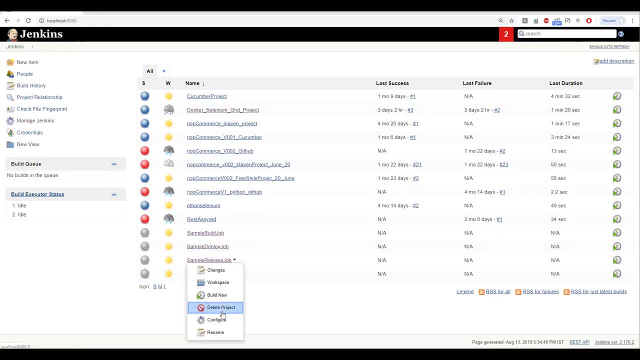 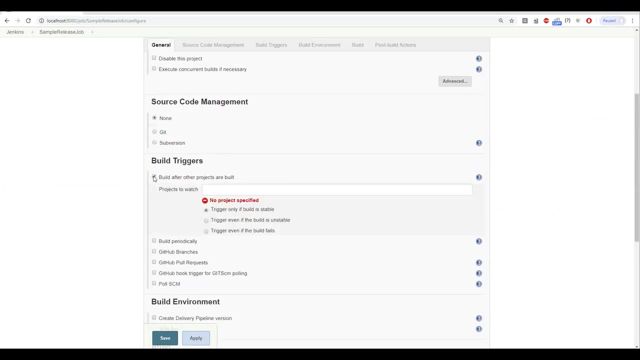 depending on testing job. now go to jenkins. i can go to dashboard. so go to the release job. so this job should execute after completion of the testing job. now again configure this. so again just come down and select build after other projects are built. now here, specify that job, sample test job. so after 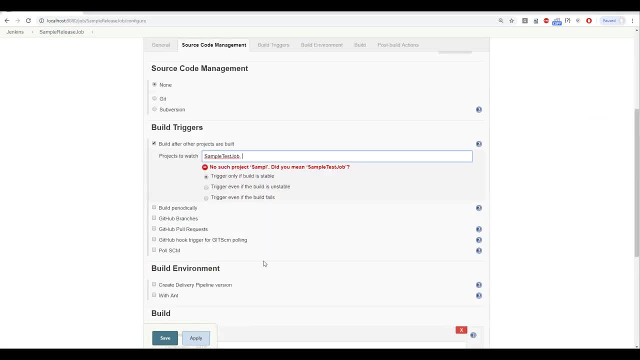 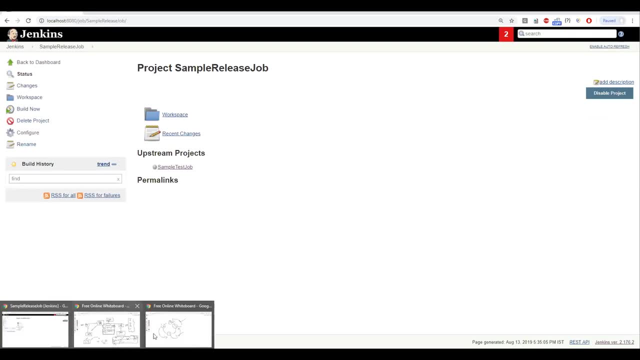 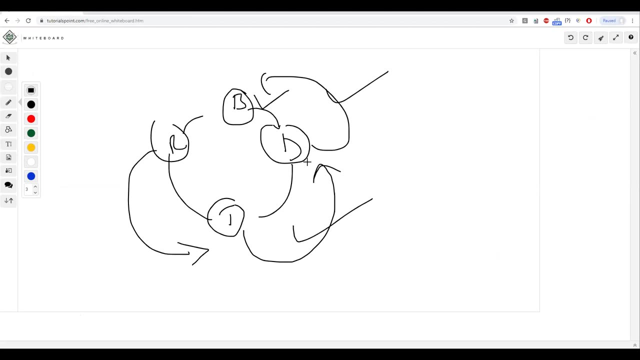 completion of this job only the release job should continue. so then apply and save. so with this we have completed the process right. so all the four stages have linked. so build is depending on deployment is depending on the build, testing is depending on the deployment and release is. 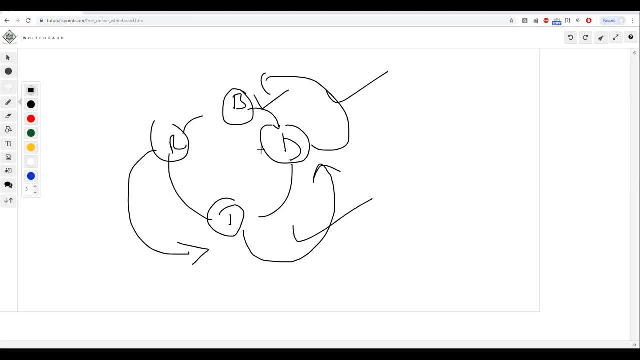 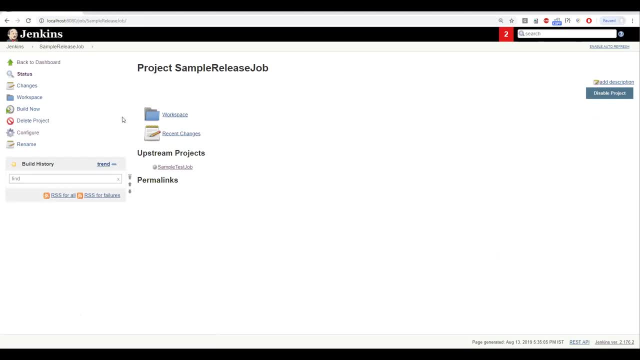 depending on the test. so everything is linked together, all the jobs we have linked. now let us see the execution part. so far we haven't talked or anything about the pipelines. okay, just we created four different jobs and i have just linked together. now, once you link it together, what will happen is 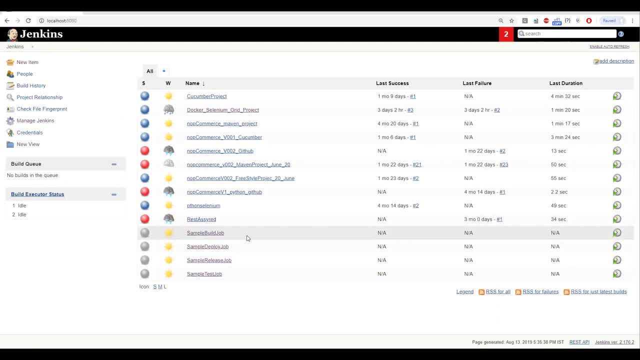 go to back to dashboard. so these are the four jobs i created, right, the first job is build, then one deployment and then test after that release. so now what happens is when i run this particular first job after completion of this, automatically the deployment job will execute after completion of. 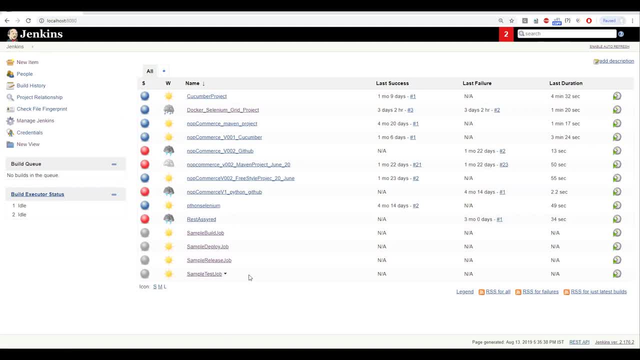 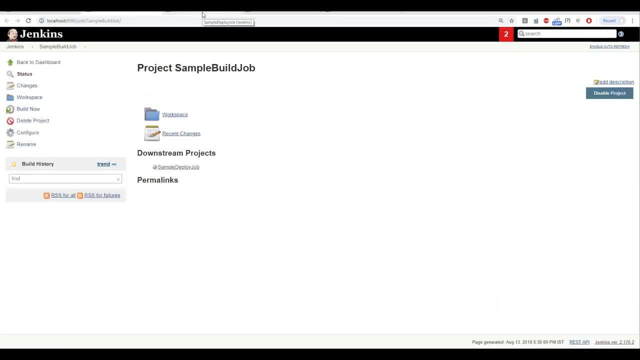 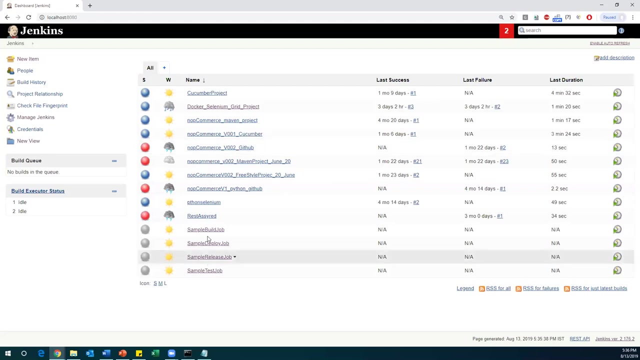 this automatically test. the job will execute. after completion of this release: job automatically executes. we no need to execute anything, okay? so let me just show you so here. i will open all the four jobs in multiple tabs, then we will look at this one. so i have opened in multiple tabs. okay, just a moment, just hold on. all right, so now let me just open these. 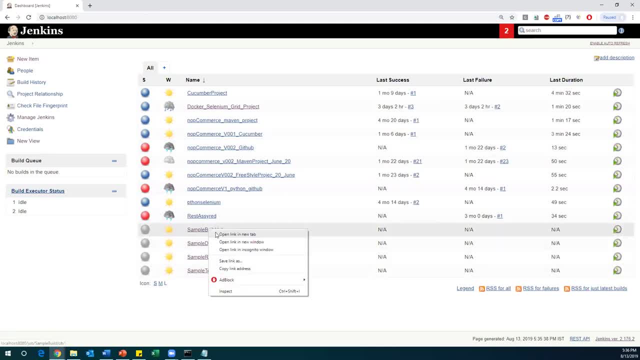 four jobs in multiple tabs. so first one is sample. this is the first job build right, so i'm opening another tab. deployment is another tab, testing is another tab and releasing, so i'm just opening four different jobs in four different tabs. now just open the four jobs in multiple tabs and then 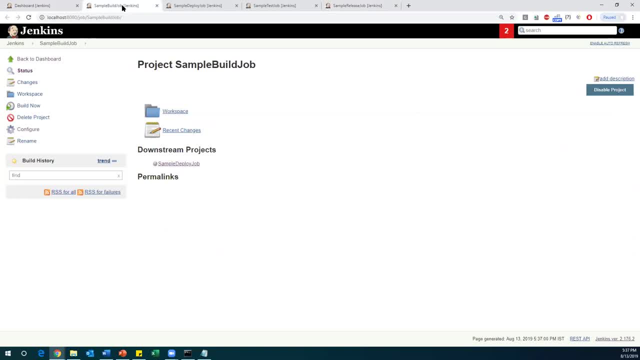 observe what exactly happening, because we already already linked together right. so now initiated- i'm just initiated- the first job that is called build job, and once it is completed, then it automatically the next deployment will job will execute after completion of this. immediately the next job will execute after completion of this tester job. then immediately release job will execute. now let's see. 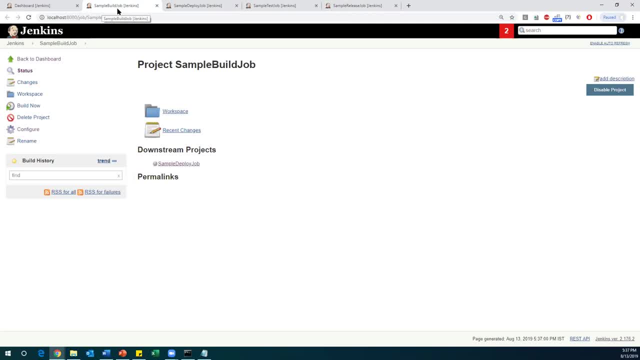 how it will work now. currently, i am running the main job. the first starting job, that is a build job, is starting now. observe what happens. so it is starting and is also passed now immediately go to the next tab. now we can see here it is still pending because the previous one still not completed. yeah, 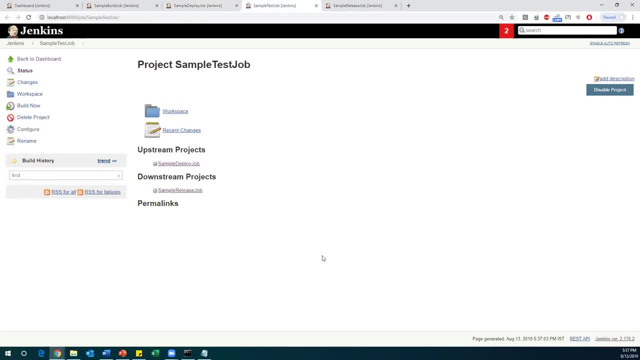 now it is started and completed. now go to the next step. so this is depending on the previous one deployment. now you can see it is saying pending. it is going very faster and it is finished immediately. it will go to the next job, next tab, and here release job will execute. yes, now it is. 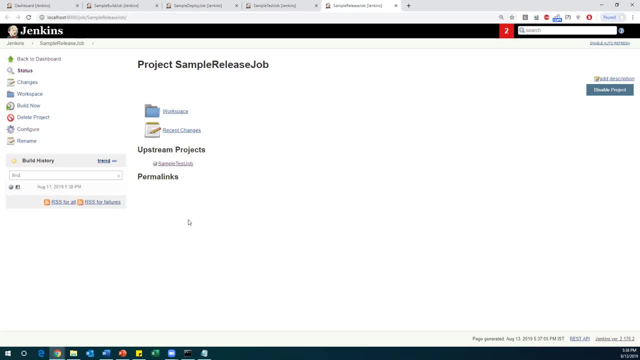 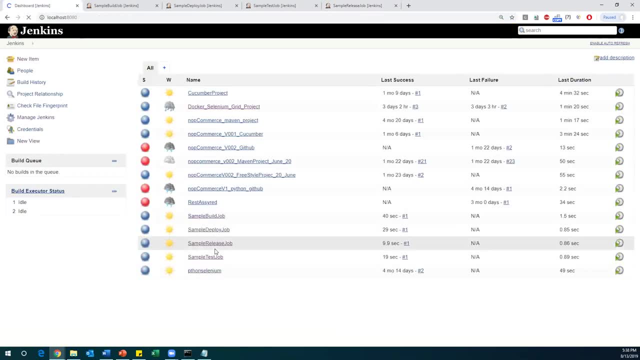 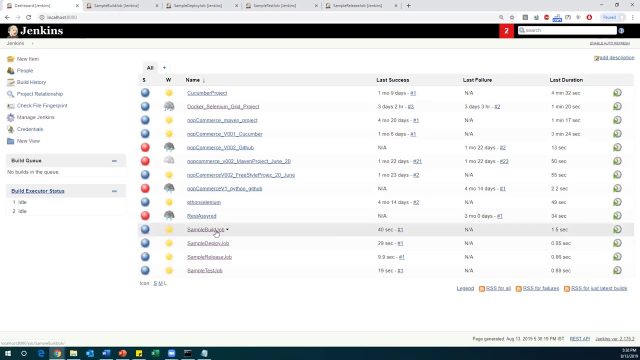 completed. right, we have just run only first job. that is a build job. now it is also completed. now go to the dashboard and just refresh here. now you will see all four jobs are successfully passed. but we haven't run all the jobs. we just ran only first job- build job- and immediately followed by 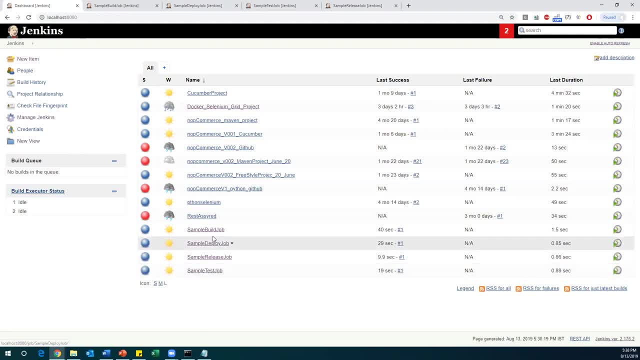 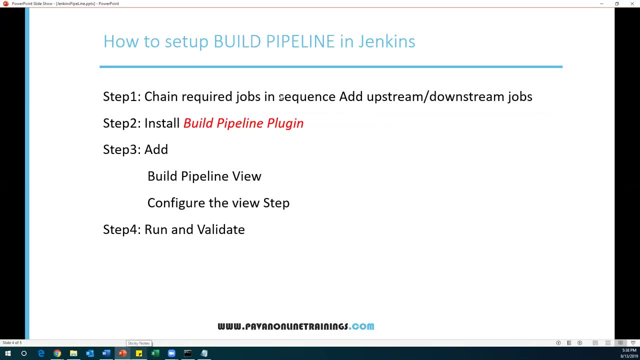 deployment, job release, job tester jobs. all those things will happen one by one because we already linked together. so this is called as a linking or we can say chain. so we have created one chain which requires multiple jobs which we need to execute sequentially. so the first step is completed. now, here, what i am doing is i am just running this. 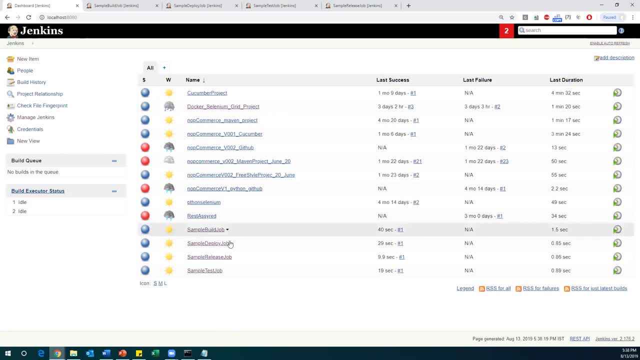 particular one build fun job. then sequentially it is going executing other stuff. right, but i don't want to do like this. i want to create one pipeline through that particular pipeline. i need to execute. okay, so now i will show you how to create a build pipeline in jenkins and through the build pipeline. 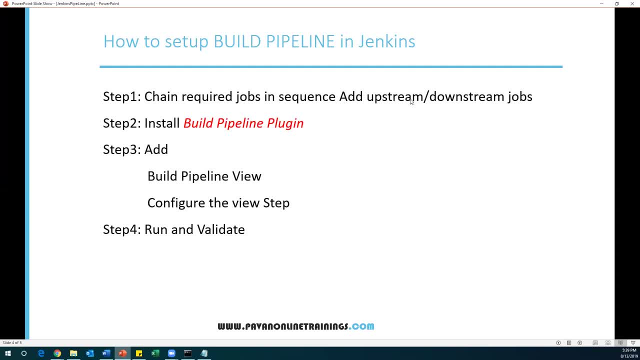 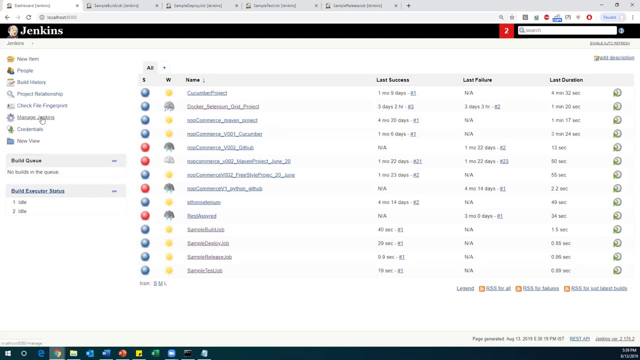 how we can execute multiple jobs as a sequential manner. okay, so we'll see that. so, to create a build pipeline in the jenkins, we need to add one plugin, okay, additional plugin which is required. so let me show you what is that plugin. so just go to manage jenkins. so once you go to manage jenkins, 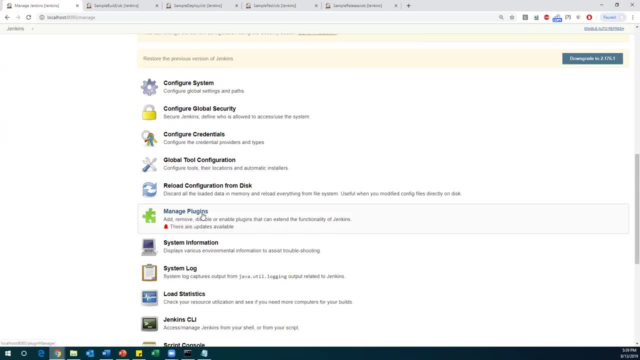 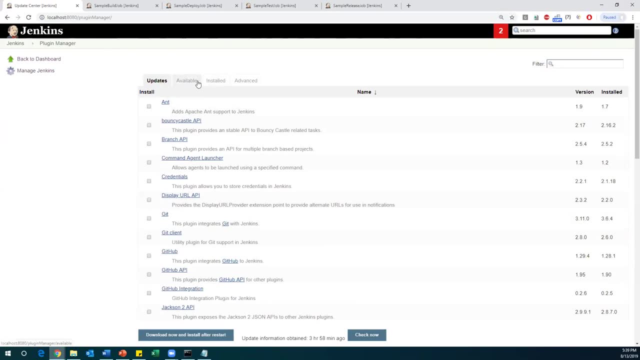 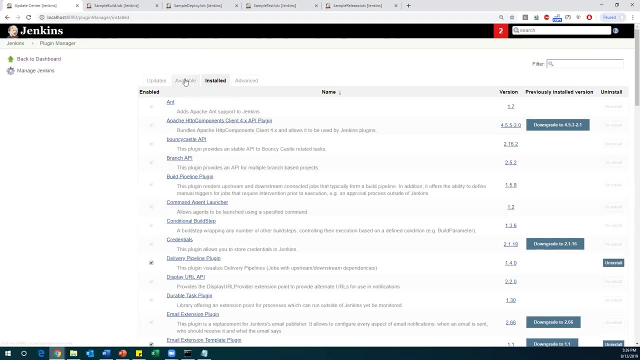 here. if you just come down, you will see one option called manage plugins. just go to manage plugins here. uh, go to available or install. if you already installed that particular plugin, so this that comes under install section. if not, it will comes under available section. okay, so under install. 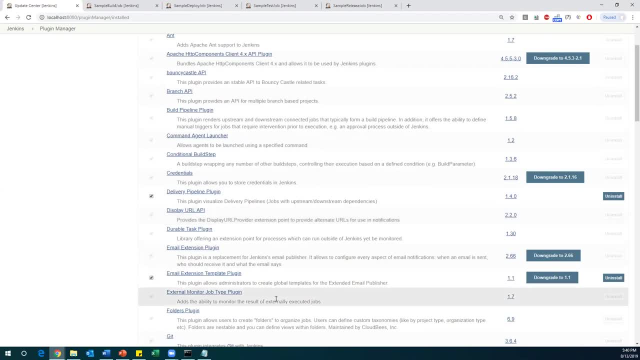 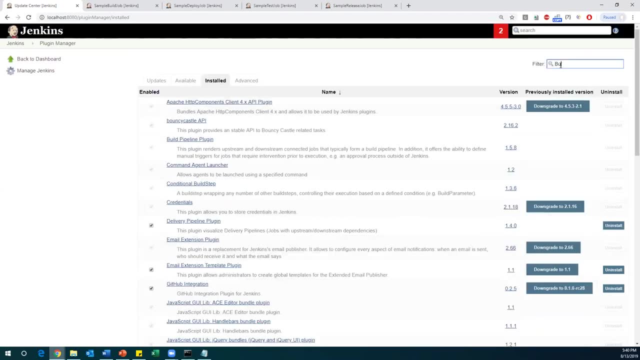 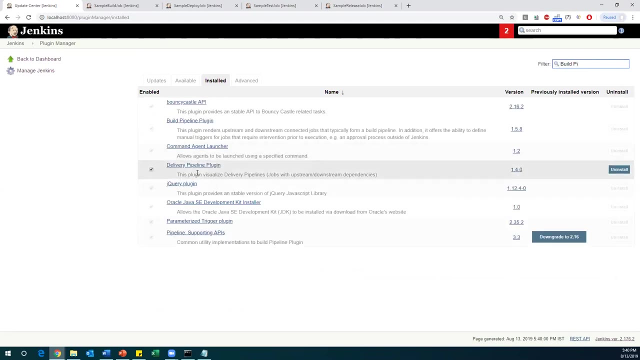 section. this is a plugin. you can see that. so here you can see. uh, let me just search for that. here i'll say build pipeline, so you can see. so delivery pipeline is there, and apart from this the build pipeline is also there. you can see here, this is a build pipeline plugin, so this particular 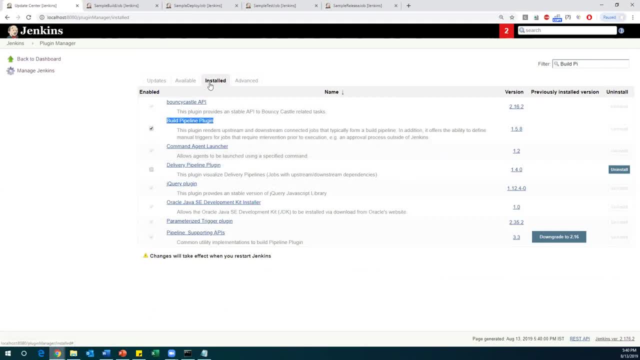 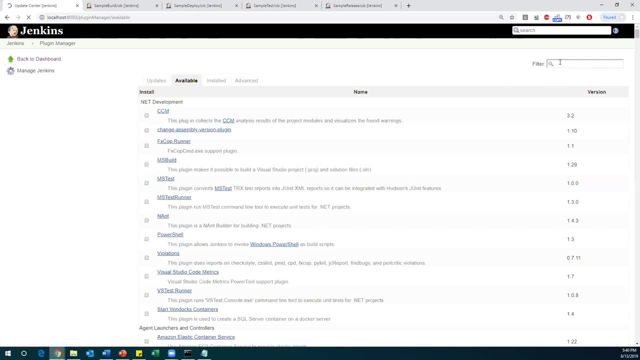 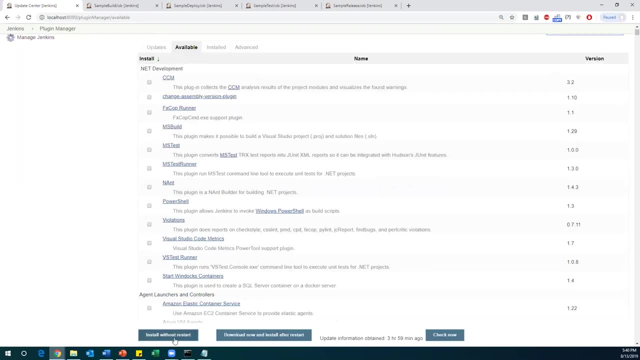 plugin you have to install because already installed here. so it is giving under installed tab. but in your case just you to go to available. go to available tab and here need to search for that. then this particular plugin will listed out here. then select that plugin and then do installation. here you can see small buttons available. 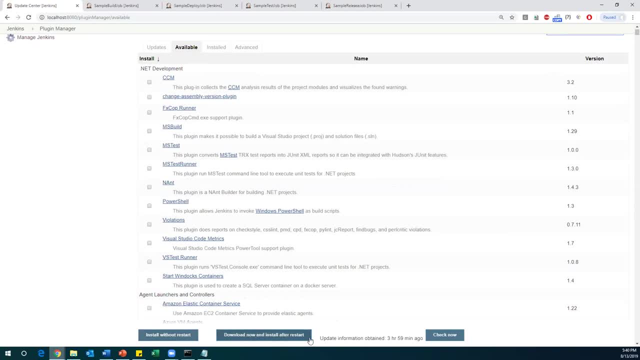 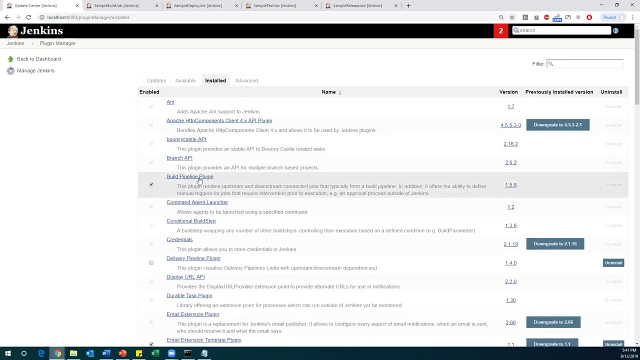 install without restart and download now and install after restart so you can use one of this option to install that particular plugin and, if required, you have to restart your jenkins. okay, so until unless you have this particular plugin, you cannot create jenkins pipeline. okay, so i already have this particular plugin, which is already installed. this is build pipeline. 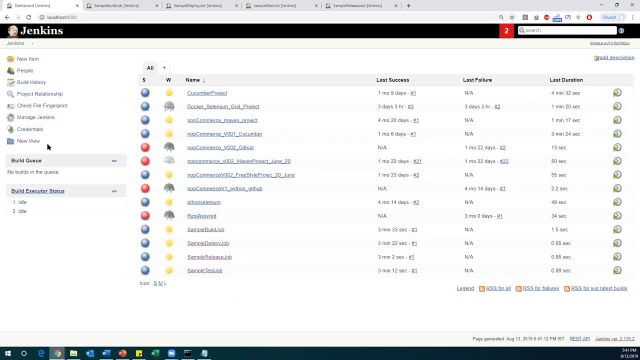 okay, once you have this, now again go to dashboard. we already have four different jobs. one is related to build process, other one is deployment, other one is testing, other one is release. okay, now i need to run these four jobs continuously, one after another, through pipeline. so how we can do that? so here i am automating the complete process. guys, there is no manual. 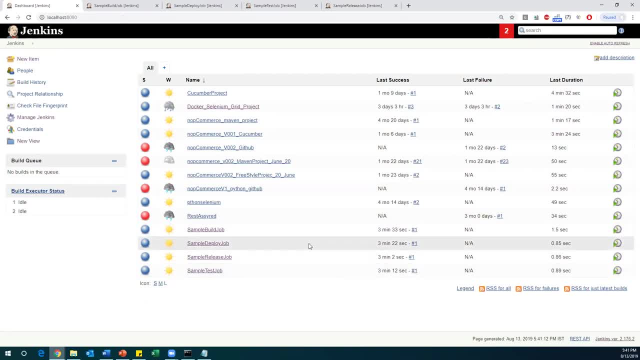 intervention is there. once we automated this entire stuff, every time it will automatically go to build pipeline. okay, so now let me just create one pipeline. how to create a pipeline? so here in the dashboard you can see one option called plus. right click on this plus and here you can see build. 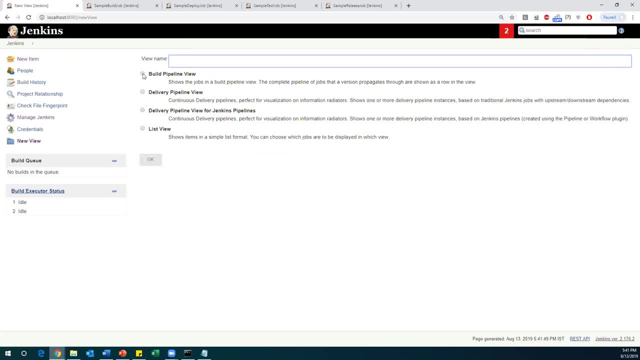 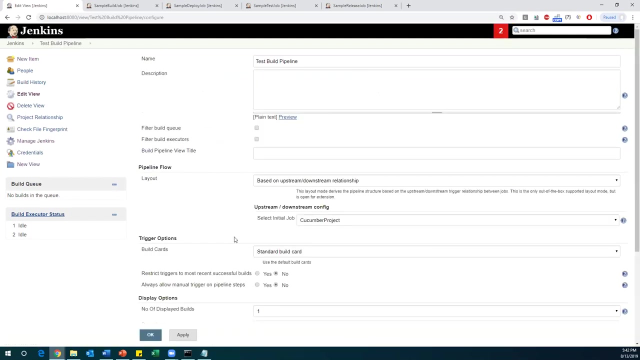 pipeline view. you can see one option here now select this one. and also you can give some name to this build pipeline view. so i just giving some name: test build pipeline, okay, so test build pipeline, build pipeline. and then okay. and now it will give you a configuration page. so inside the 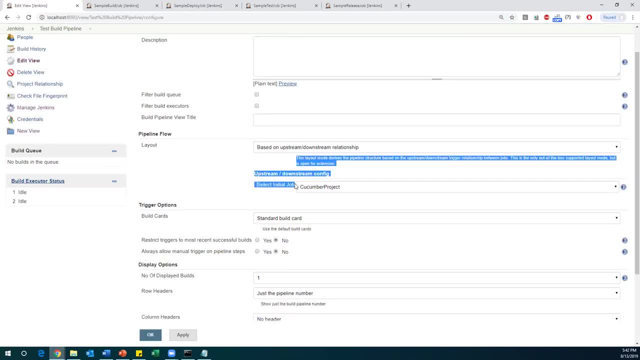 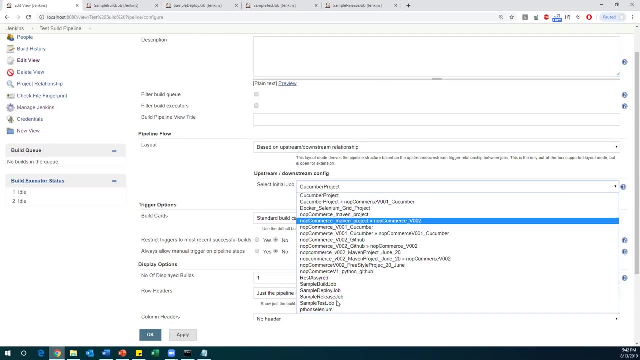 configuration page. you have to select the initial job so you can have all the description and prerequisites, and here you need to select. there are so many jobs are already created in your jenkins earlier, right. so where we need to start? what is the starting point? so the starting process. 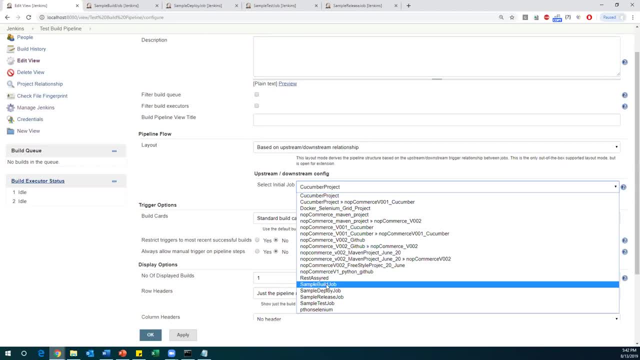 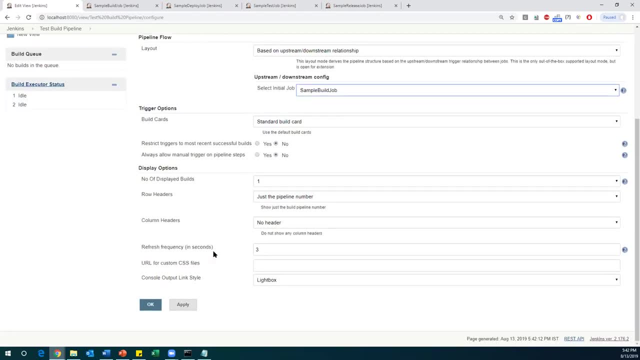 is a build process. so sample: build a job which we have created. so we need to create a build process which we have created. so now we need to select this. after selection of this, just come down and you can just display number of displayed builds. you can also increase this number. 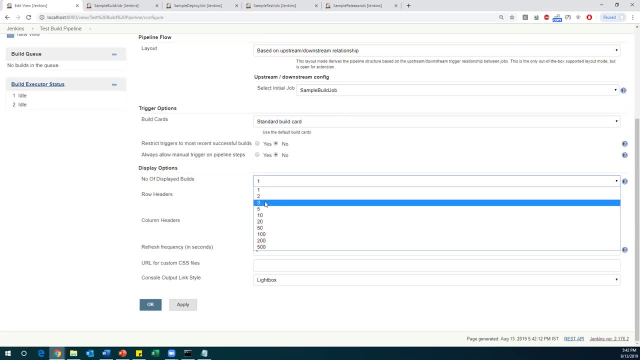 okay, let's say three to five entries. what is this? one is number of displayed bills means how many times you have run will be displayed. i'm just selecting for now five or three, five is fine, and then apply then. okay, now i have done. okay, now you can see it is body. 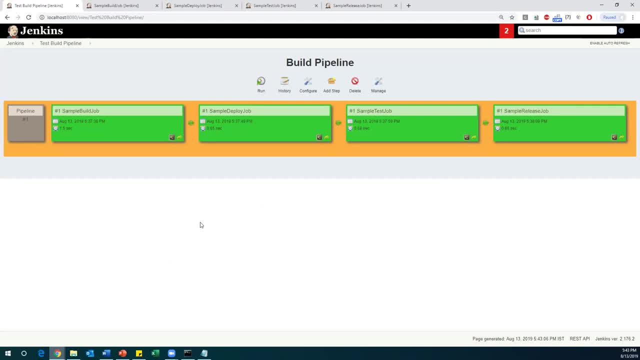 what it is showing: build pipeline. okay. so what is this build pipeline contains? you can see here we have run all the jobs only one time. right, we have linked together only one time. so the first one sample build job is executed successfully, then sample deployment job executed successfully. 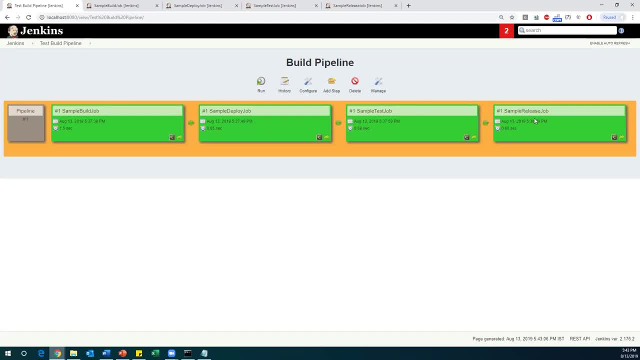 then sample test job executed successfully, then sample release job executed. so now all the activities are part of your pipeline. so this is called as a pipeline. so build by line. so all the jobs now part of this particular pipeline, so you no need to run them manually now. 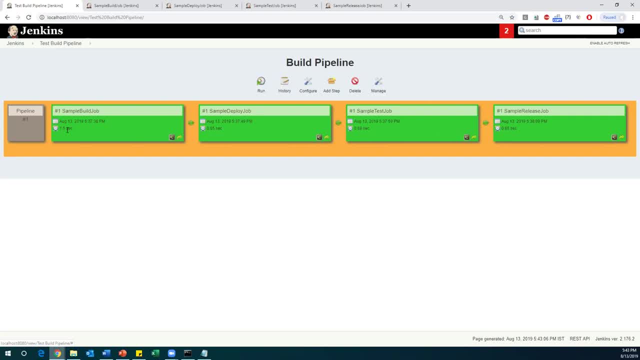 so just you need to run this particular build pipeline. all the jobs will run one after another. okay, this is one round of execution. we already done so. it is showing here. now let me just run this build pipeline. when you click on this run option, it will go and execute one more time. i am 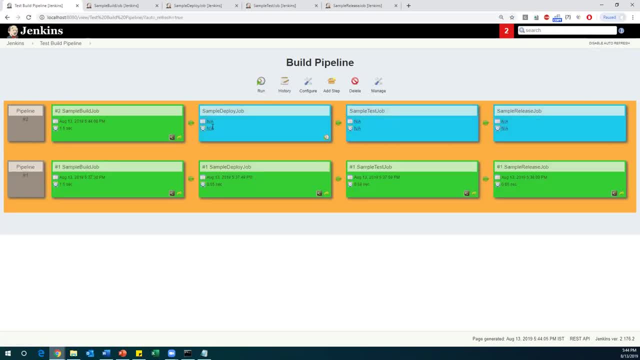 enabling auto refresh so that we can see that now we can see there is one more entry which is created. now the sample build job is running. after refreshing the page, then again one more job is executed. next and next. now currently the blue color is representing in progress. 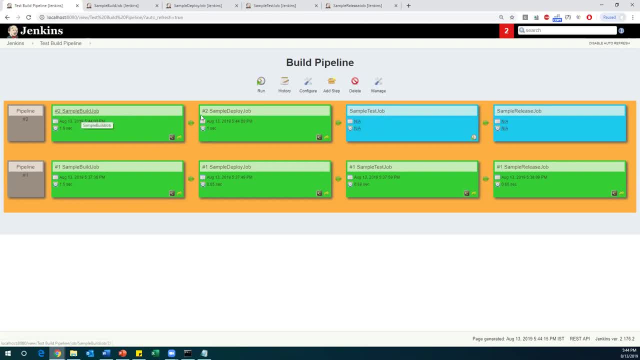 so one and two, these two are completed. so build a job and, uh, deployment job is completed. after refreshing you can also see: yeah, now testjob is also completed. now, finally, release job should execute and successfully pass now once you've done another refresh, so you will see, sample job is also. 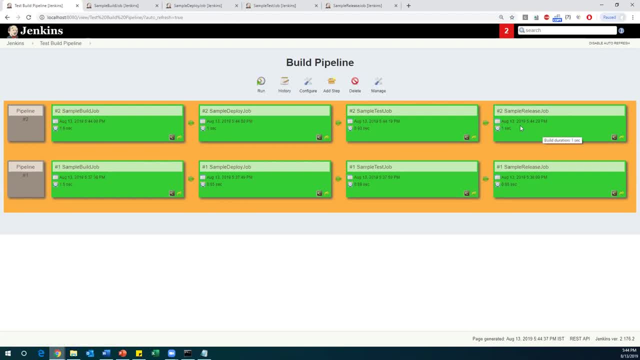 completed. so totally all are green means everything successfully passed. if somewhere something is failure or some job is got failed, it will come inside the in red color. okay, so this is how we can create a pipeline and we can execute all the jobs in sequential. okay, so if i run one more time, 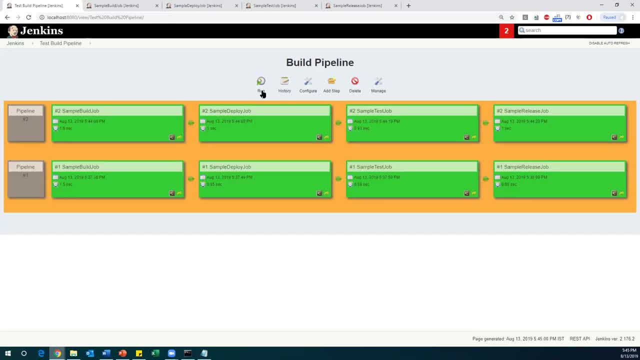 so just click on run one more time now again. it will create one more entry pipeline. three now again. all the jobs will execute one after another. now it is again refreshing my page. we just enable the refresh automatically. this will refresh. now we can see the third round is. 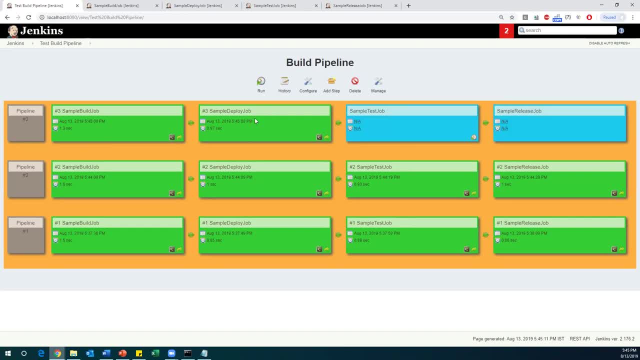 started and build a job and deployment job is already completed. now testing job is in progress. after that, release job will be executing. now release job in progress. now the release job is in progress and once it is done, our complete process, continuous delivery process, is completed. all done, so now third line, third round, is also. we have created and done okay. 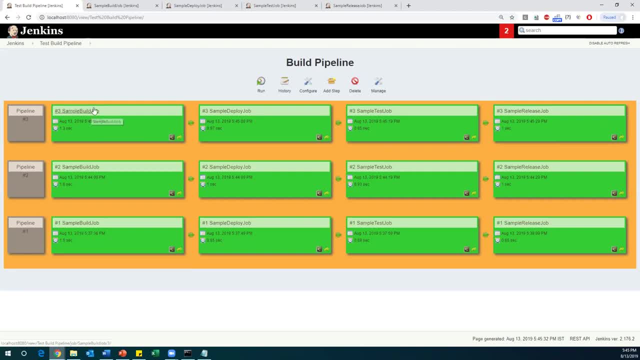 so let's see how we can create a pipeline and automate all the processes, so build, process, deployment, test and release. so here i've just taken very simple example to demonstrate how we can create a pipeline and how we can execute the jobs, but in the real environment, every job 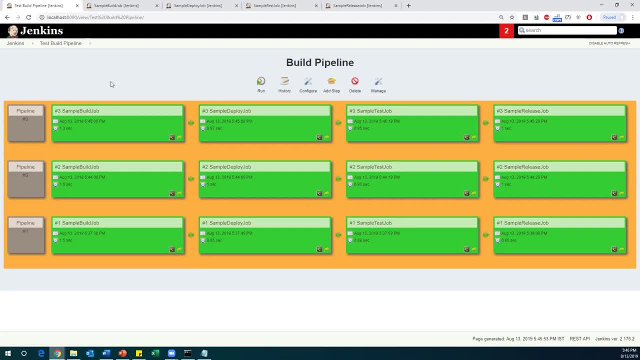 contains lot of stuff. so every job will do lot of things internally. they will run lot of commands to build the job, okay, deployment of the build and testing and releasing process. so in every job they to run a lot of commands but at the end they will integrate everything inside the pipeline. 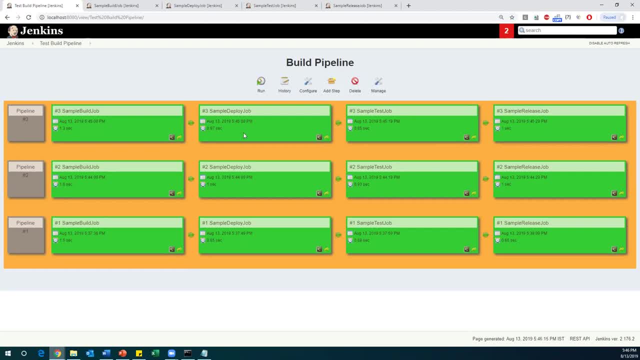 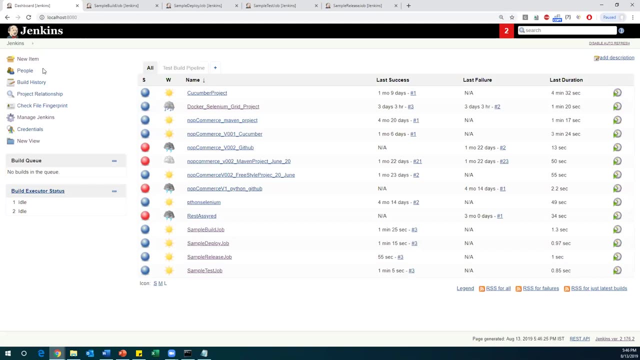 and every time they just run the pipeline and automatically all the process will go on. so this is called as a build pipeline. so again, if you just go to back to the jenkins, so just we have seen build pipeline right. so like this we have one more pipeline can be created. that's called delivery. 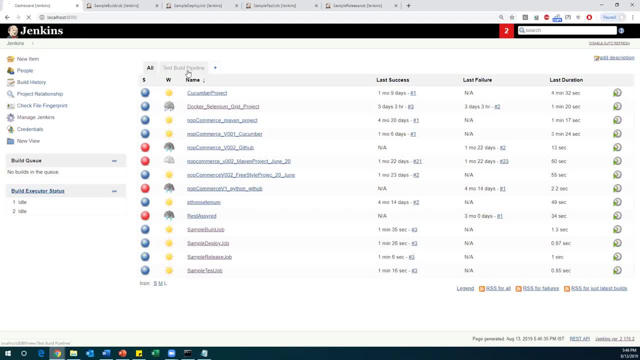 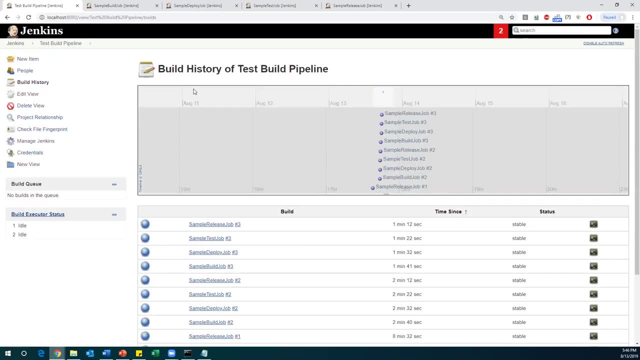 pipeline and here, if you just in the build pipeline, we can just run this. we can see the history. we just go to history. we can also see how many times we have run this, how many failures we have, and also we can see a lot of information. we can also configure, we can also add one more step. 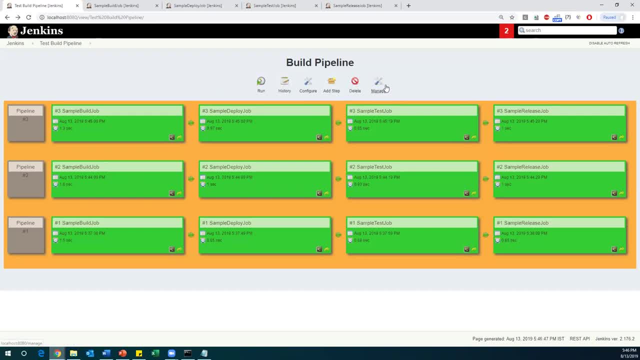 we can delete that one managing a lot of activities. we can do that. suppose. if there is any job is somehow it is getting failure, then we can still rerun only that particular job. we just have this particular option rerun. if i click on this rerun, what happens? again? this only. 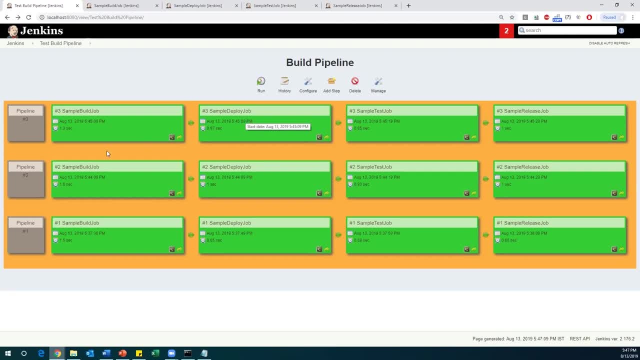 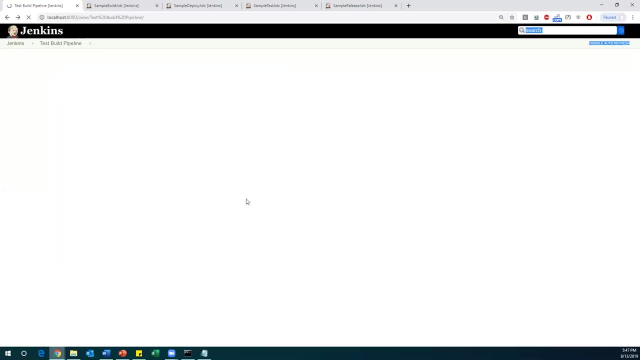 this particular job will execute one more time. and if you want to see the output of each, every job, you can have a console window here. if you click on the console, it will show you the console and you will get exact message here for every job. you will get the console window here. you can see the output of. 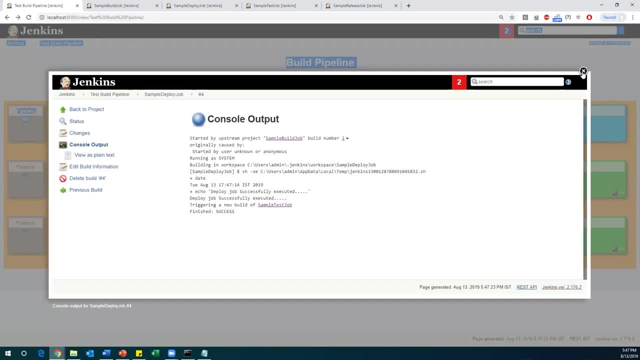 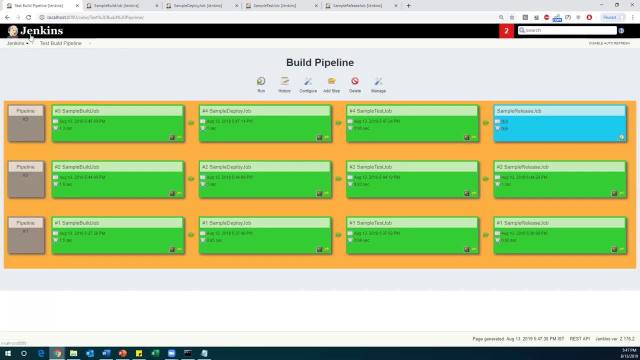 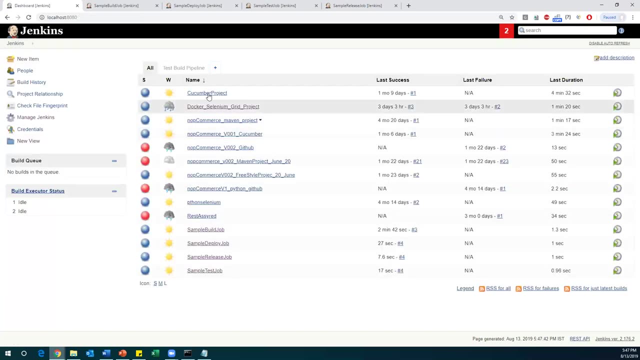 the particular job also. okay, so here itself we can manage everything. and this is a build pipeline. so there is one more type of pipe pipeline we can create, that is delivery pipeline. so now i'll show you how we can do this. so here just click on this tab and here this time, select the 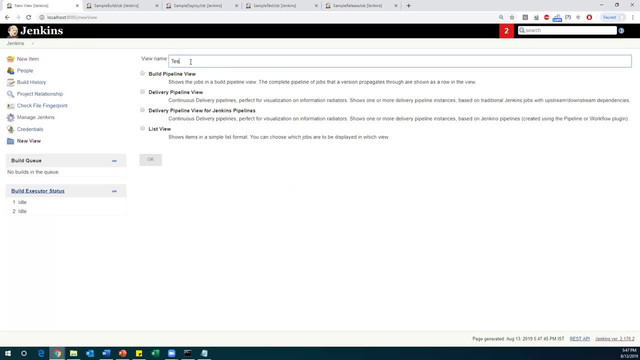 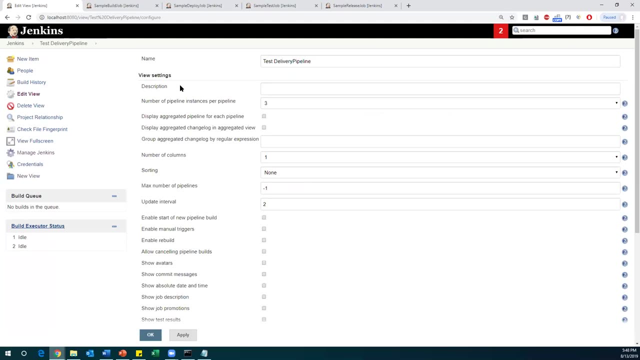 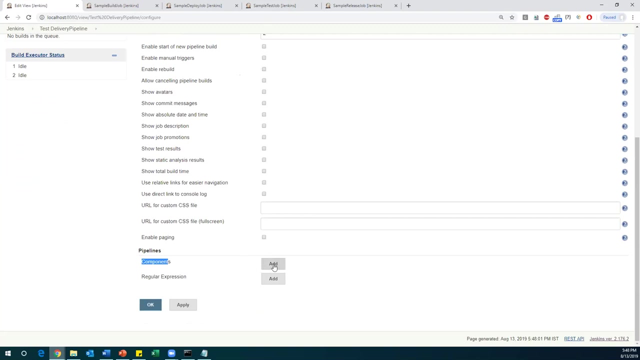 delivery pipeline view. okay, so our name is as test delivery pipeline pipeline delivery pipeline. so just select uh. delivery pipeline view, just click on. ok, it is just like a report. now you can have a default options, as it is just come down here. pipelines components: here we need to just click on add now. here we need to exactly specify what is our. 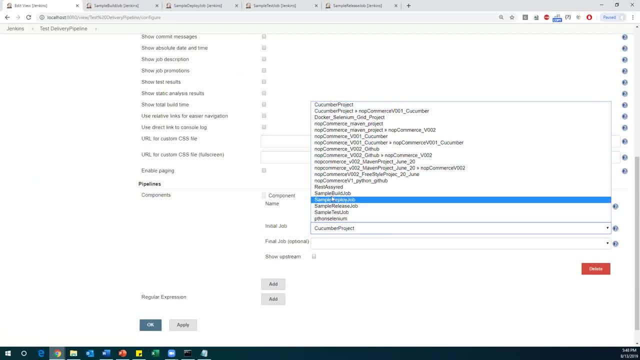 initial job from where we need to start. so creation of sample build job rights. this is the first job. sample build a job is a starting point. now, selectors, if you want to give some name, you can give it. so I say: my delivery pipeline, okay, my delivery pipeline. so it just gives some. my delivery pipeline demo- okay, just give. 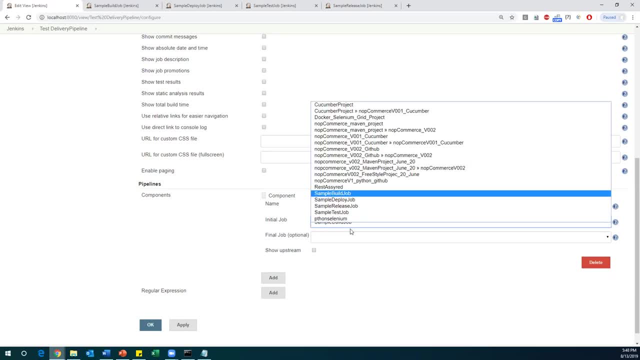 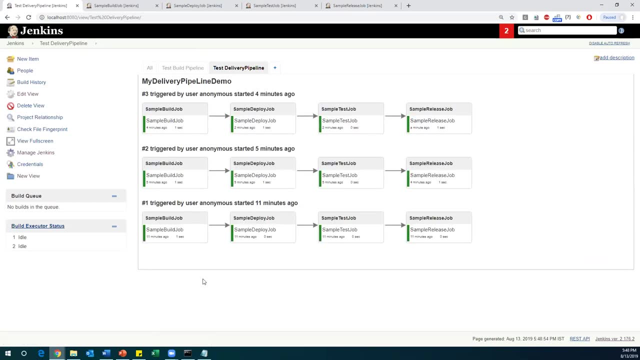 some name to this- and here need to select exactly where the initial job should start and after that apply. then okay. once you click on ok, now we can see you. it will show you the complete report here. so how many runs we have done earlier? three runs, one, two, three runs we have done now. all the runs, all the. 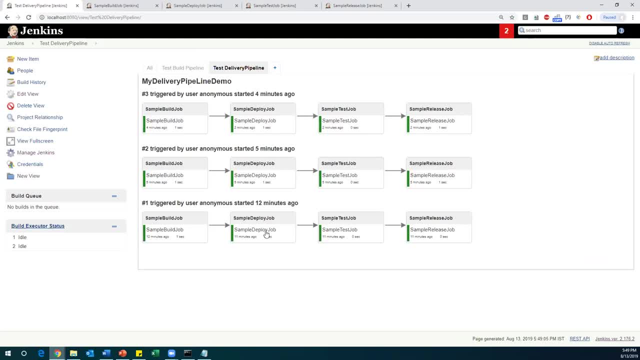 complete sequence is executed, see: build a job, deployment job, test job, release jobs. in every round all the jobs have been successfully executed. so this is a delivery pipeline and is a built pipeline. okay, now I can also go to delivery pipeline. you can see this input or this can also view this in beautiful. 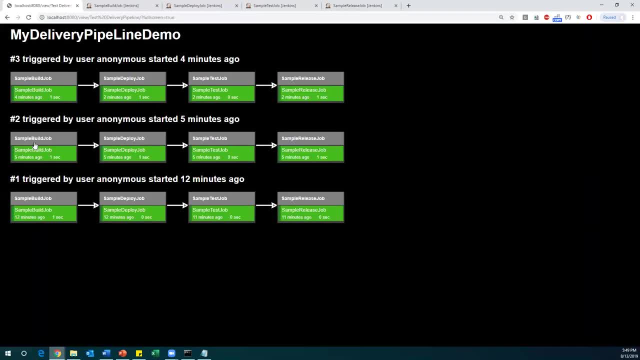 manner. you can just go to view full screen and it will give you like this and you can see in every round all the process, how it is goes and where exactly it is get. but here you cannot run anything. just it is a visible. so just a presentation. okay, just 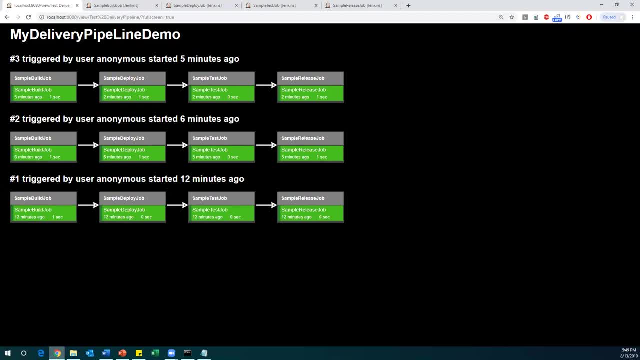 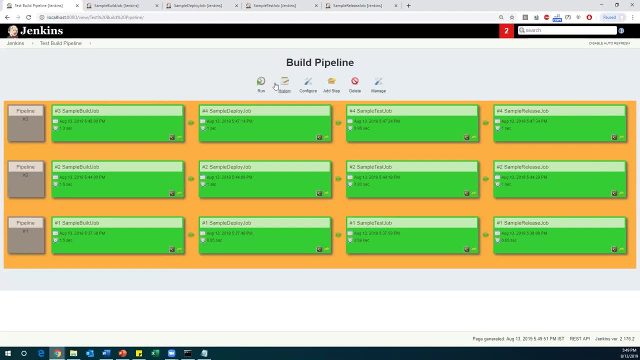 visualization so, but you cannot run and configure nothing. you cannot. this is just to deliver report. but if you want to run the complete pipeline, then go to test to build a pipeline and you can have few options here. click on run again. one more round of execution will start. you can see the history. you can do the 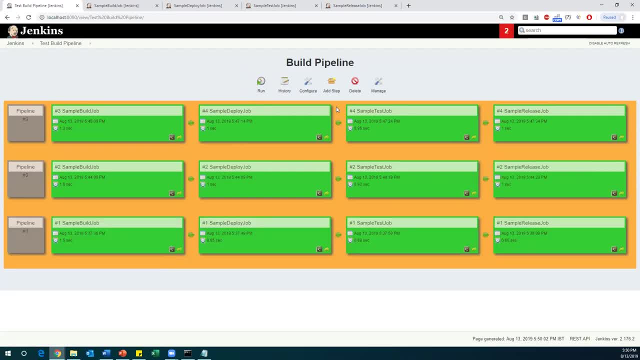 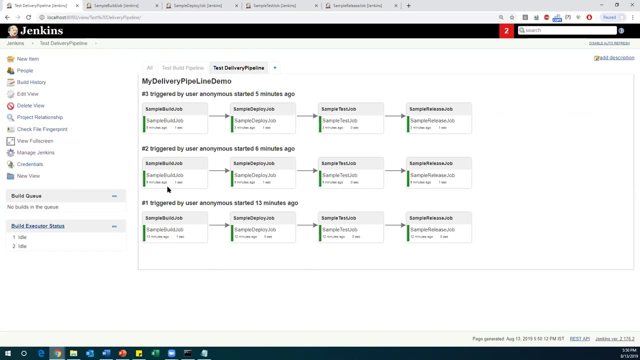 changes in the configuration. we can add one more step, or if you don't want anything, we can just delete it, and lot of actions we can do in the build pipeline. okay, so in the delivery pipeline we can just see the report like this: right, so this is a basically concept of pipeline. so in this video we 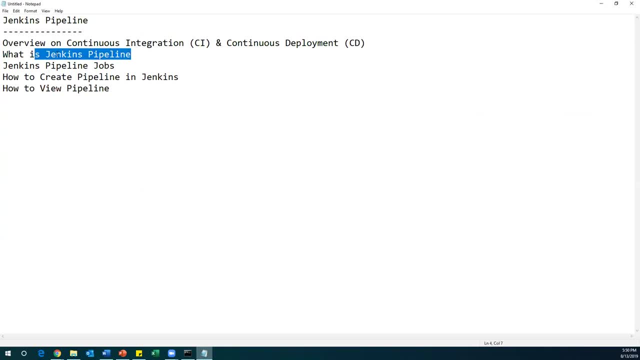 have understood what exactly Jenkins pipeline is, what is pipeline, jobs, and a pipeline means it contains multiple jobs and how to create a pipeline in Jenkins. and then, finally, we have seen the pipeline report right. one is build pipeline, the other one is delivery pipeline. okay, so this is all process.